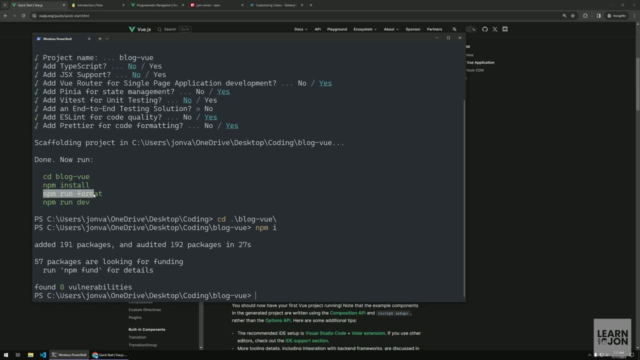 or install. There we go and we don't need to run this one, because it will format the files which we don't need. We are going to delete them anyway, but what I want to do- install. run the last command: npm, run dev. This will start up the local development server so I can open it in a new 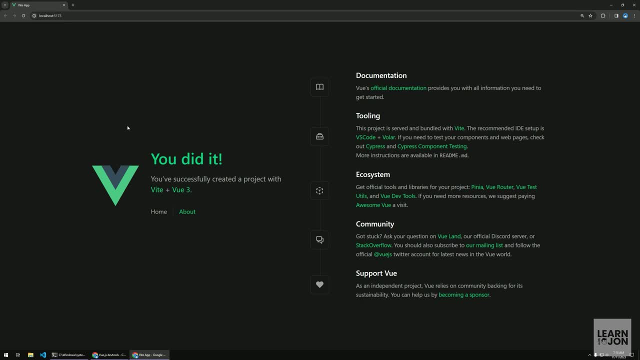 browser and see what's going on here. So this is a boilerplate of a Vue application When we install it with npm. so, and because we are using Vue router, we have two routes by default. I would recommend installing this extension on your browser. Vuejs dev tools and I believe it. 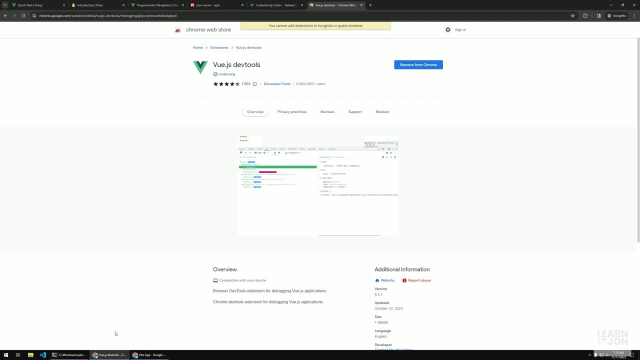 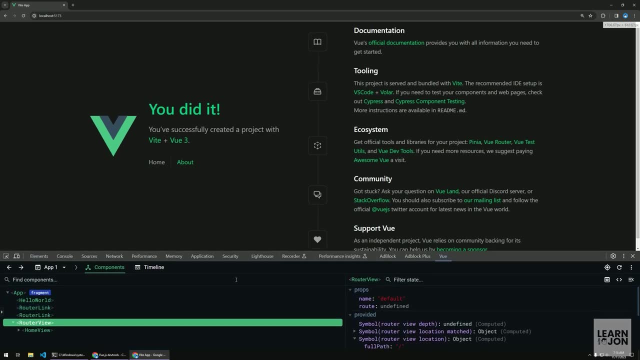 is available for Chrome and Firefox. I don't know about other browsers. When you install it and inspect a Vuejs application website, you can have this Vue tab in your console or developer tools, or whatever we call this one, and this will give us a nice overview of the things, of the components. 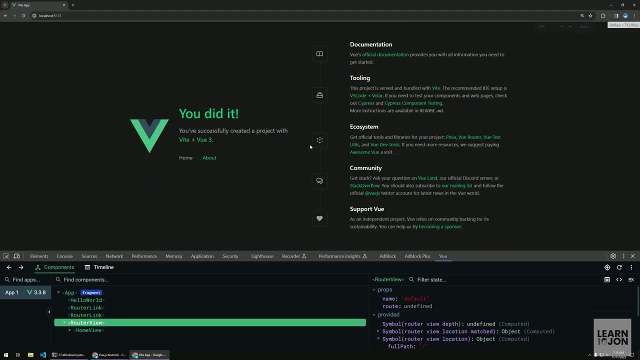 as you can see here, as the of the components of a Vue application, We have an app component which is the root of our application and every Vue application must have a root component and within that we have hello, world, router, links, router, view. These are part of Vue router, which I will explain. 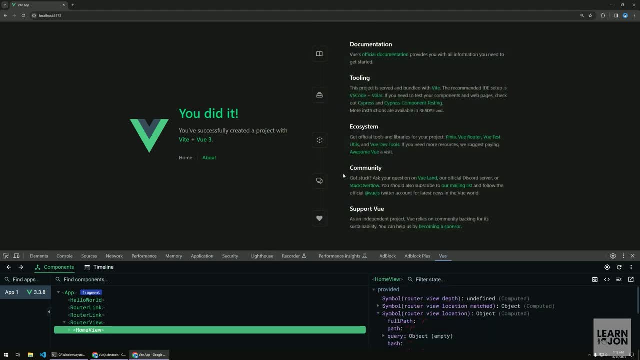 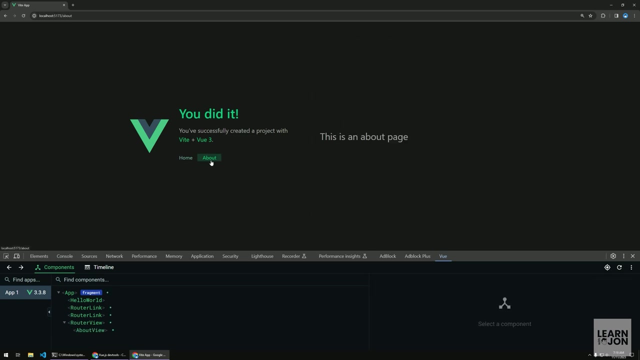 later and then you can see we have a home view on the right and within that we have nested components and it goes deeper and deeper. So all of these are different components and we will learn how components. but watch what happens as I click on the about. This home view will change and, like that, 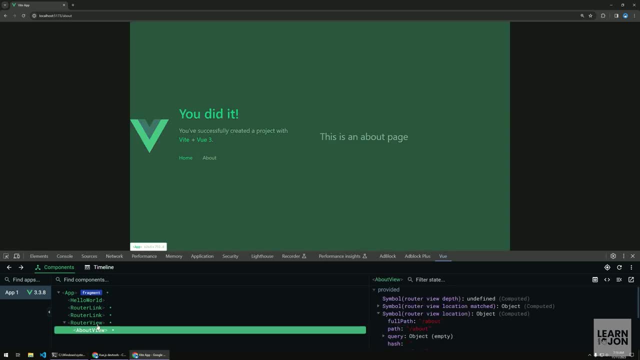 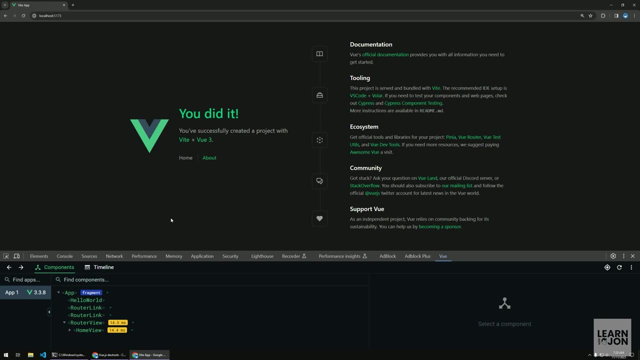 so you can see, I just changed the component using this router view or router link rather, and this is basically a component based model that Vue offers, which allows us to build single page applications, so we don't have to render the whole page every time something is changing. We can just go back. 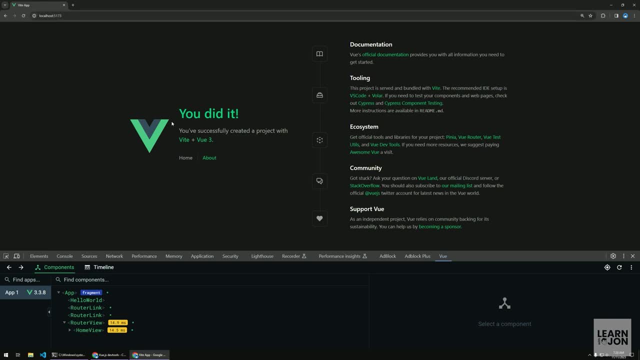 and forth just like that, without any call to the server. So basically, that is a single page application and doesn't call the server every single time. It just gets the information needed from the server on the initial load and then the client handle all the changes, which is in this case Google Chrome. 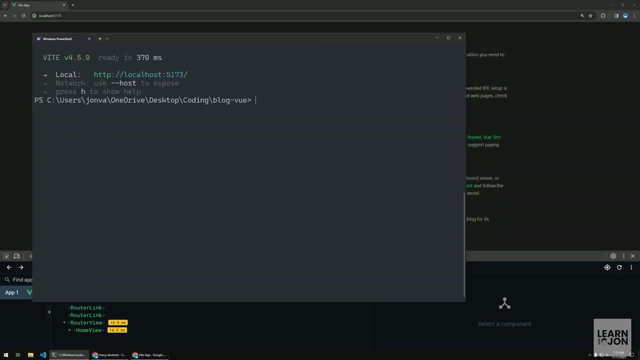 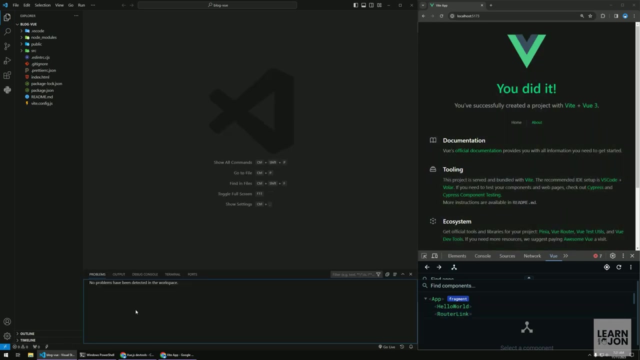 So let's go back to the terminal here, and I'm going to break this local host by pressing ctrl c and I'm going to open VS Code by pressing, by typing code: space dot. There we go, All right. so I put these side by side and I'm going to close this welcome and for now we are not running the local. 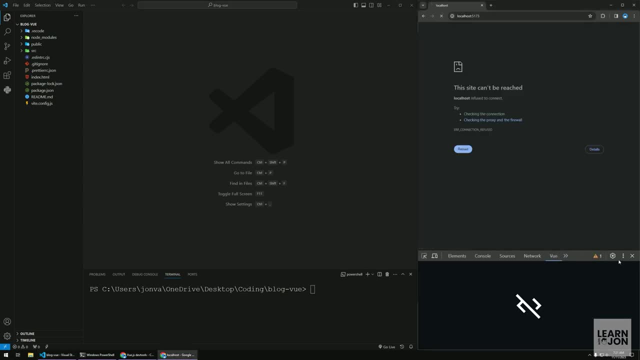 server anymore. so this will break. if we refresh There we go. That's okay For now we're going to leave it like that. Let's talk about these folders and files just for a second. We don't need to know what's going on here, but some of them are quite important, like this indexhtml file, which is again. 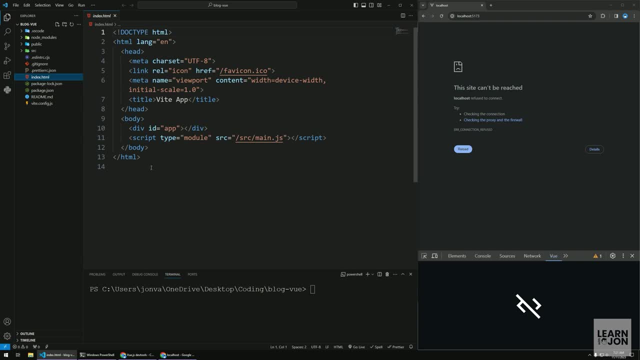 the root of any website, whether they are web applications, whatever they are. So every website has this indexhtml and that is the root where the client browser is going to read it and notice we have a div with the id of app and this is the wrapper. 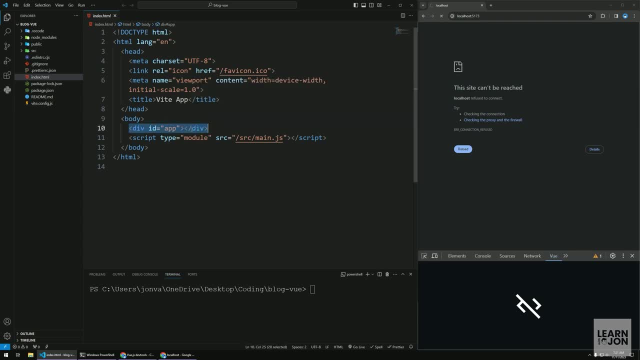 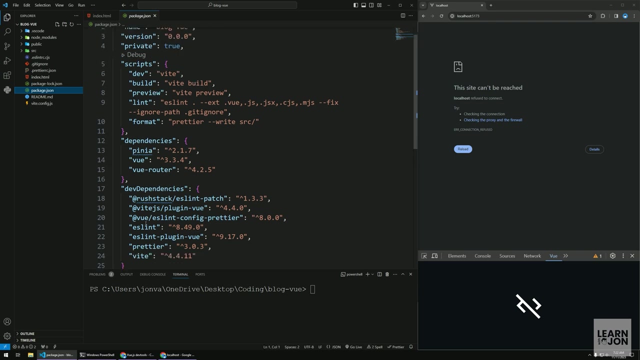 Of the view. so all the view components go within this wrapper. so this, we can consider this one as our root. and then, of course, the script tag where we are saying: read from mainjs in source. We will go through this in a second. We have our packagejson which lists the information about our 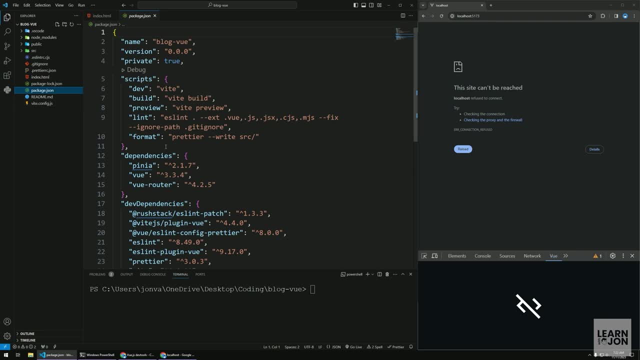 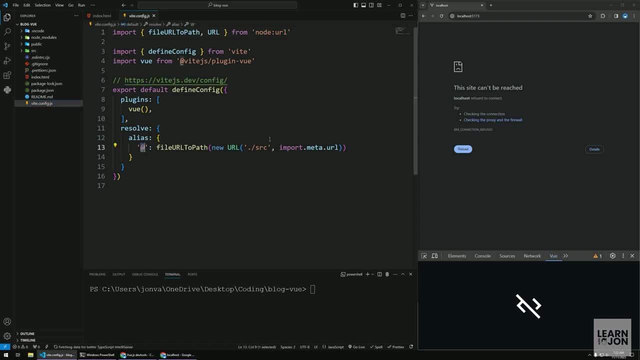 project, the version, the dependencies, the scripts and yada yada. So we have this vid config. we don't need to touch this one, but this is some configuration for our project so we can use LESS, for example, like this one, when we want to Address the source folder again. we don't need to touch this at all, and the rest is just some. 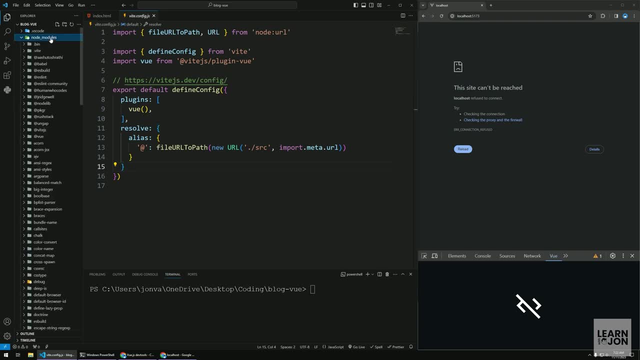 configuration. Within the folders we have node modules again containing all the modules related to our project. we don't need to touch that at all. We have our public folder that everything that is public is going to go in this. so like this icon on top of the title page and anything that could. 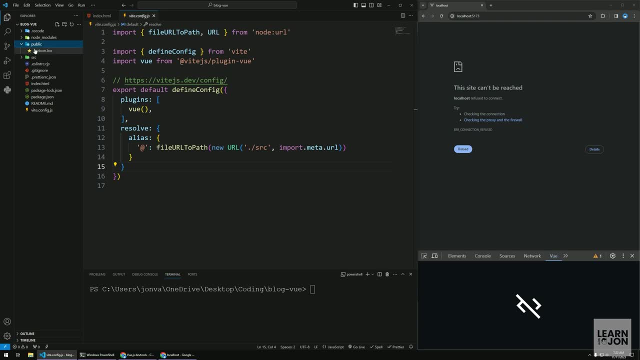 be public goes in here. So nothing too fancy and in fact we will delete this one. we will make our project as clean as possible. Now, the source folder is the brain of our application, so whatever we do, it's in here, and you can see that mainjs also is in the source folder, So within the source. 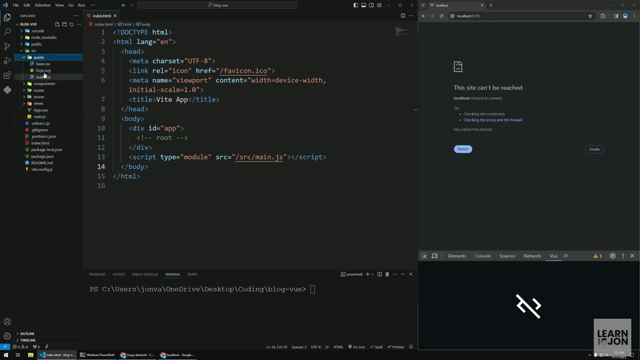 folder. we have assets folder where all the assets like css, icons, media or whatever we have goes in here and we can grab them from assets folder. so we have a clean, organized code and we have our components. as the name suggests, all the components go within the components folder, like remember. 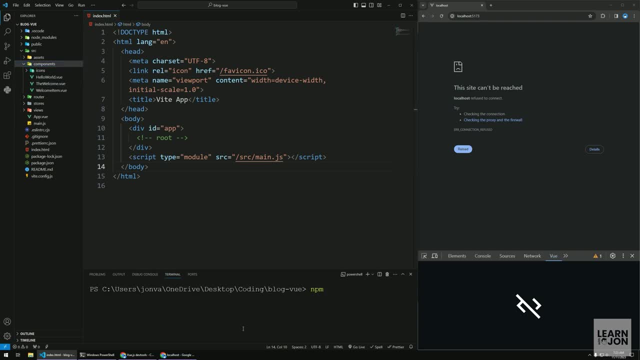 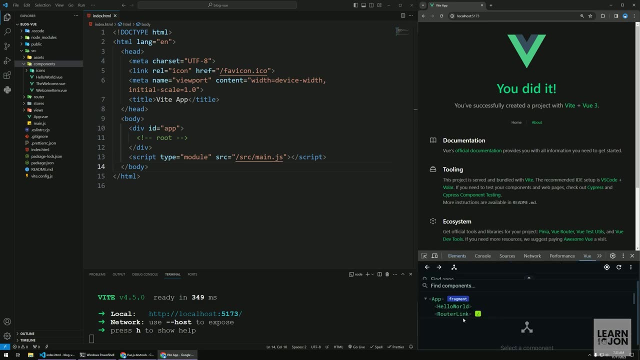 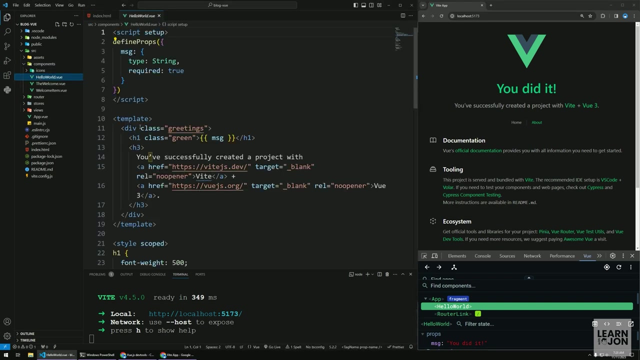 when we inspected this site. let me run npm, run div, so we can have it here and let's close this one and it again, because that didn't work. go to view. there we go, so you can see, here we have this hello world component, for example, and it comes from here. from this component we have that div with a class of 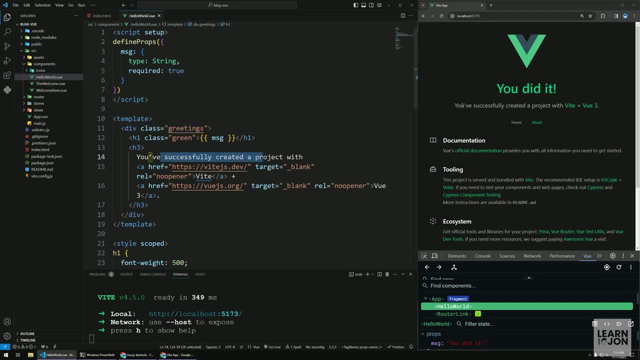 greeting and it says: you've successfully created the project. there it is, and again, this is a bit at first, because we're just getting things started. it could be confusing, so we will delete all of this. we will start from ground zero, but to just show you these components on the screen, they're all. 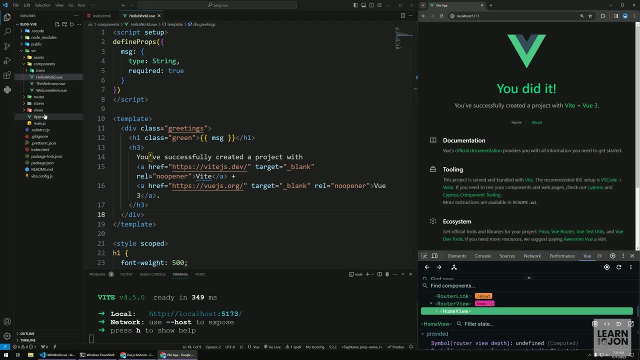 coming from this folder. so we're going to start from ground zero and we're going to start from ground zero, but to just show you these components on the screen, they're all coming from this folder and they are injected into this app component, which is, again you can see here, this app is the. 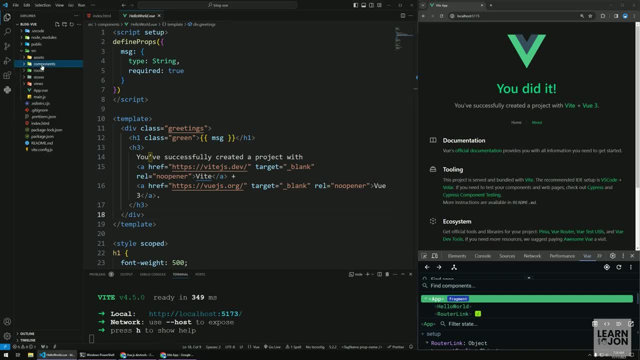 root, so everything goes within here anyway. so that's the component. router is, of course, the view router and we're not going to touch this one at first because we will cover the basics and then we get to the router. but we will clean it up. the stores is pinia and it is for our state management. 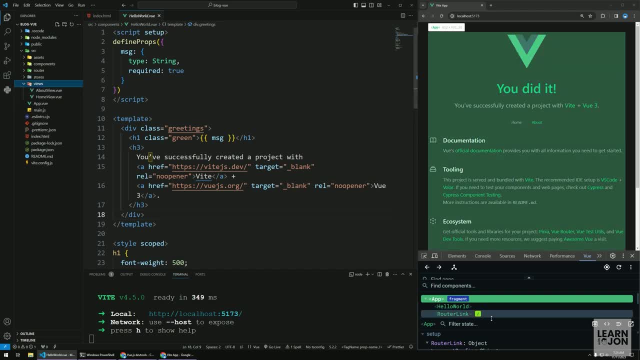 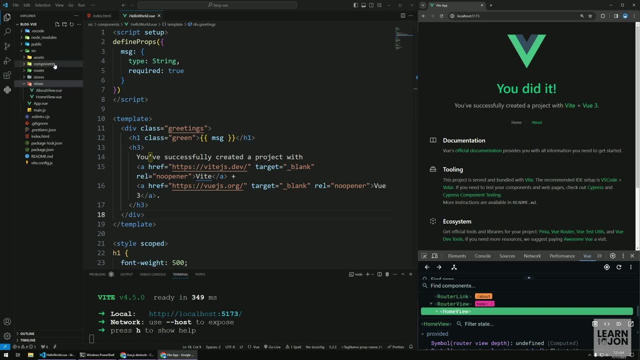 we will get to this one as well later. and the views, of course, are these main views. if you will, a view, think of a view as a page and a component of the children within the page. so we have an about page and a home page, or in this case we call it view. so those are the 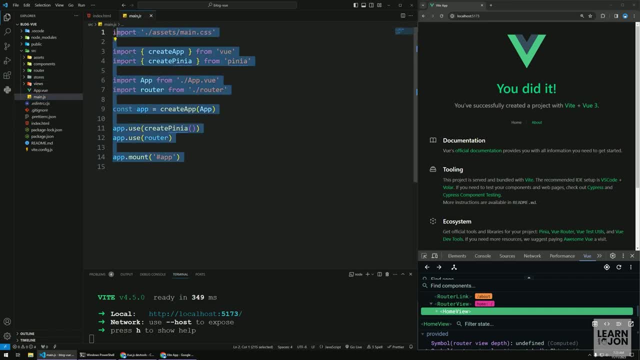 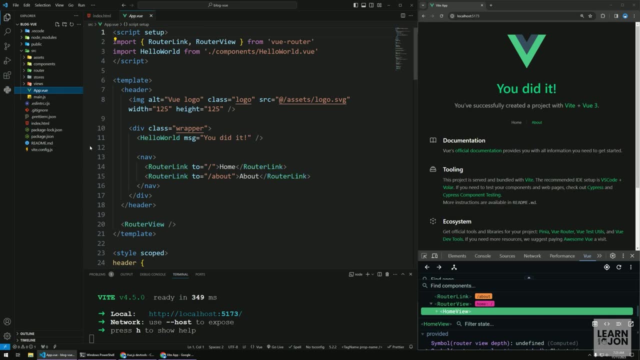 folders and, of course, we have our mainjs, which is the root javascript file, and then our appview, which is the root component of our application. now, you notice, we have we are using the view extension and this is because we are using a build tool and this is a single file component. so 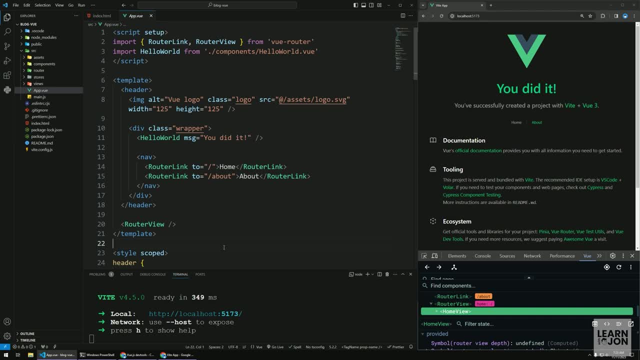 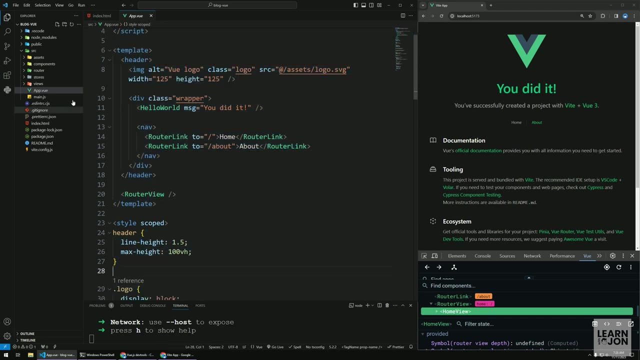 this is one of the features of vue js that gives us the ability of a single file component and that basically means we can have all the logic related to one file or one component within one document. so we have a script tag, we have html and css, just like any website. imagine every component or every. 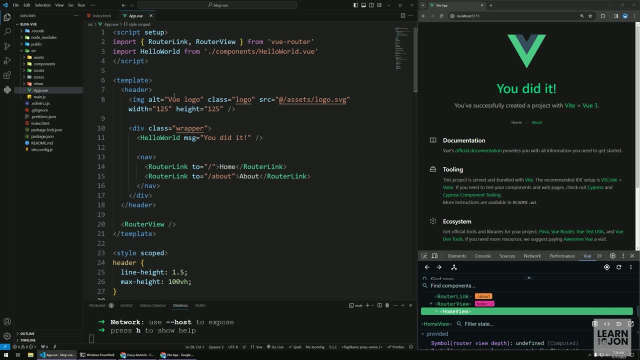 view extension file is its own html file with all the dependencies in it. for example, you can see in the app view, which is the root of our application, this hello world from the components that we saw before, which was this part right here. so you can see we are importing it from that folder and we are showing it just like an html. 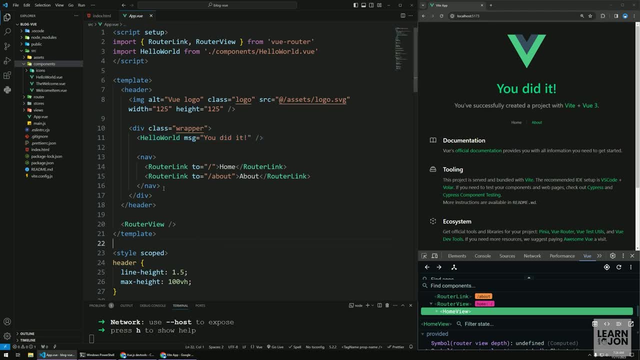 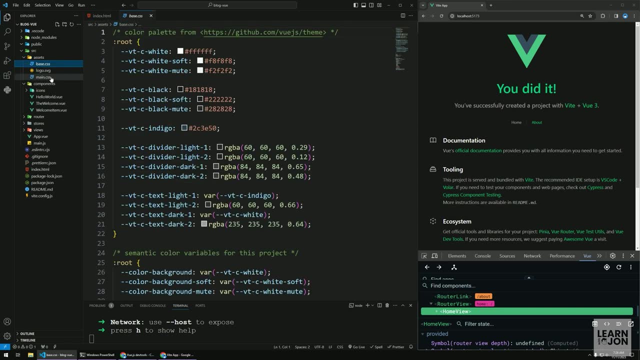 tag on the screen. all right, before we get any further, let's do a cleanup, okay. so let's clean the house, and i'm going to start with public folder and i'm going to delete that icon within the source folder. i'm going to go into the assets and delete everything. i will add my own css and 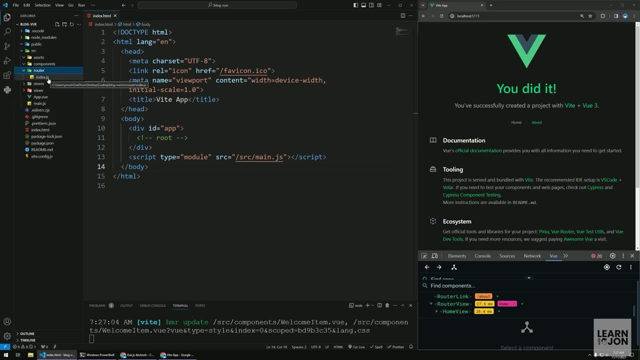 within the components, i'm going to delete everything too. router: i'm going to keep it, but inside the indexjs, within the router folder, i'm just going to delete this about object, right here. i only need a home page for now, so i'm going to save this one and we will. i will explain this when we get to it. we are getting error, that's. 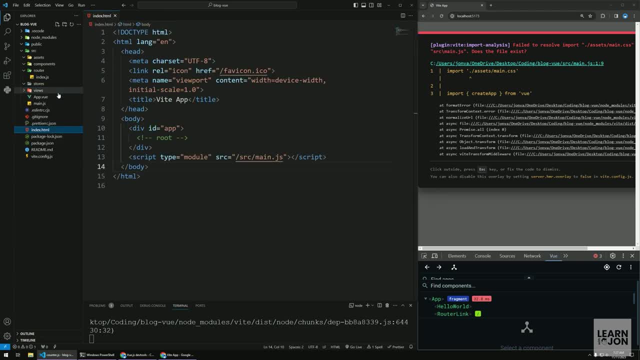 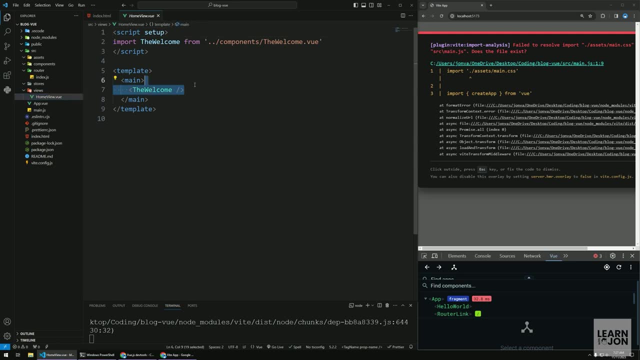 fine, because we are deleting things. so, stores, i'm going to delete this counterjs. we don't need it. within the views, we can delete the about view because we deleted the route. within the home view, we can delete this welcome because we deleted the component right, so i'm going to save this one. 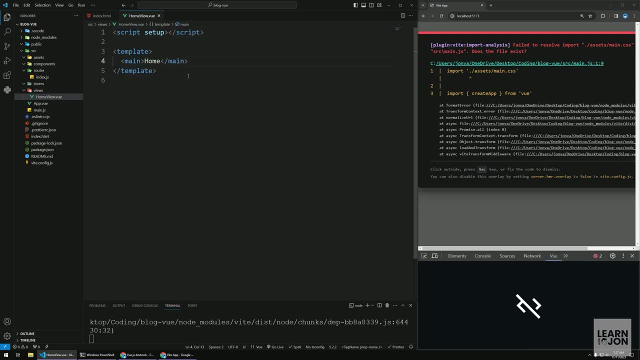 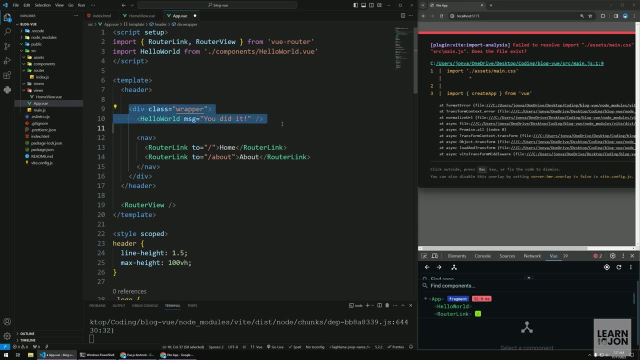 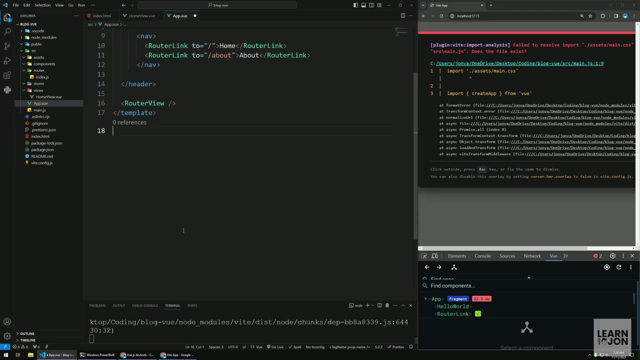 too, and i'm just going to type home here so we know we are on the home page within the app. i'm going to delete everything except the nav, so keep that header on this div, this div down here and the rest is there. this import up here and all the styles don't need it. 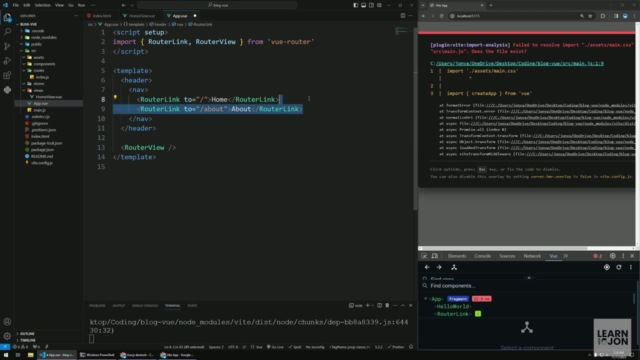 and i'm going to format the code so it looks better. also this router link, because it doesn't exist anymore and save. so again i will explain these router links and router view, because these are part of view router, so we're not there yet in the mainjs we can delete this maincss. 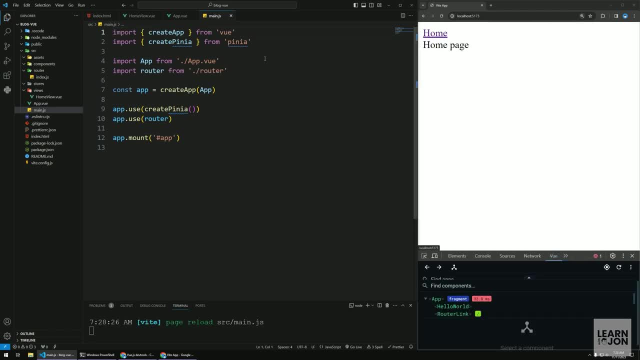 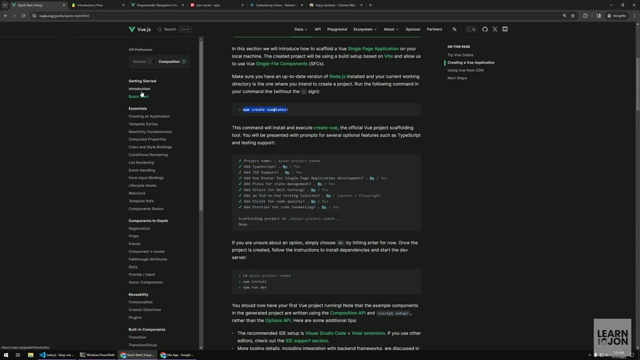 we're good, save there we go. so just one link and one text on the page, nothing else. oh, one more thing: indexhtml. we are still using that icon up here, this link. let's delete that one too. now, we're good, i'm going to close everything except that mainjs. so in viewjs documentation, if we go to creating. 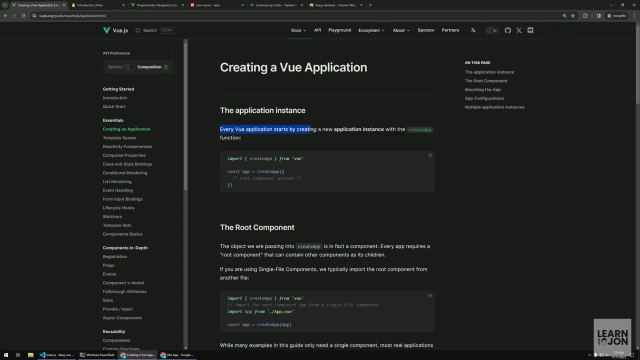 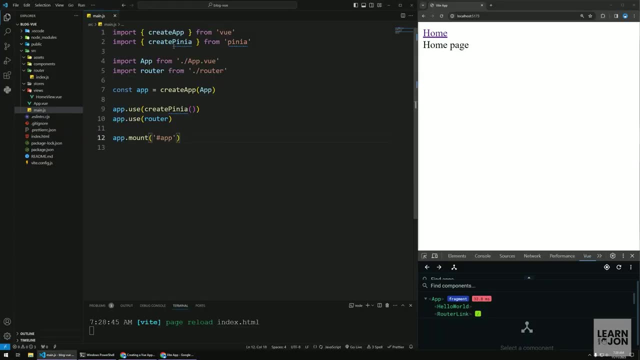 an application here you can see, that says every view application starts by creating a new application instance with the create app function, this function from view, and you can see here we are importing create app from view. this is the root of everything. this is the root of a view. 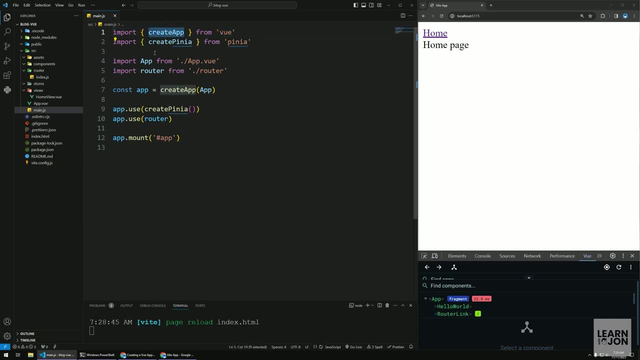 application. we start from here, so we are importing create app and then passing this app, which we are importing from this appview. so this is our root component, like i said, and we are importing it and adding it or passing it into this create app function because this expects a component and this 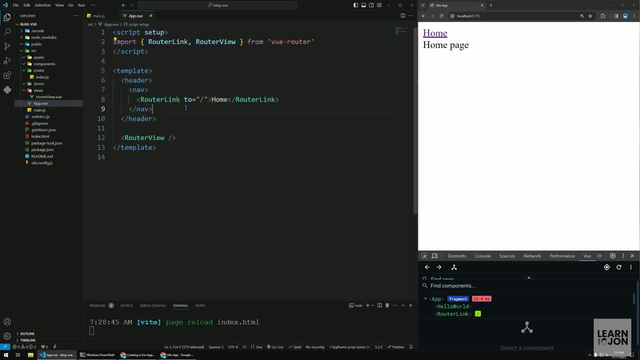 is our main component. you can see there's nothing special here except this router link. oh so, if for a second ignore these router links and router view, you can see there is nothing but html here. so that is our root. and then when we pass that root into the create app, we need to mount it. 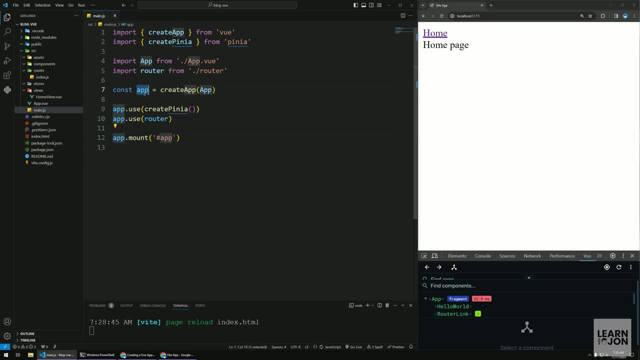 into the dom and the mount function on the app. it will ask for a wrapper for a css selector. so where do you want to mount it? we already said we want to mount it within this div. so if we put anything outside of this, this is just going to be simple html. nothing regarding view. we also have 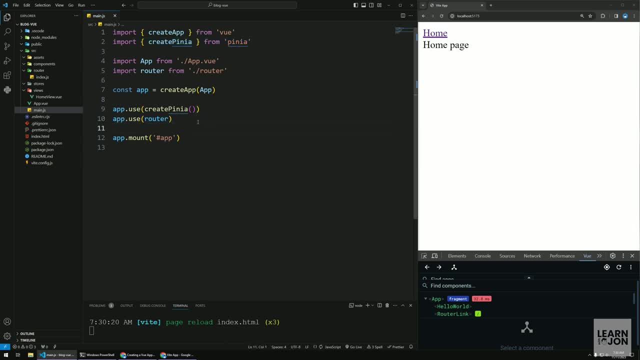 create pinia and view router, because we're not there yet, but it's quite clear what it does. create pinia: it's bringing the method that pinia needs to run its logic, and then we are telling our app to use these functions or these plugins. and again, when we get to it, we will talk about these. 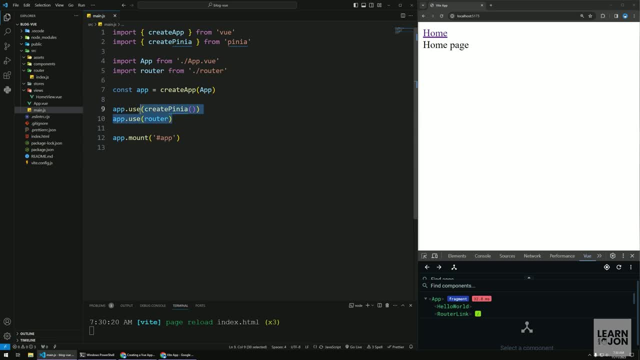 things. for now, we're just going to focus on the view application itself, not these plugins. all right, i'm going to go to home view and use this home view as our playground and i'm going to close out here in a minute. let's talk about the way we get our portals to this environment, to this. 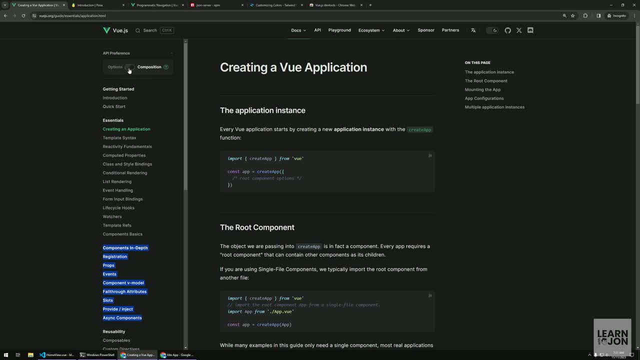 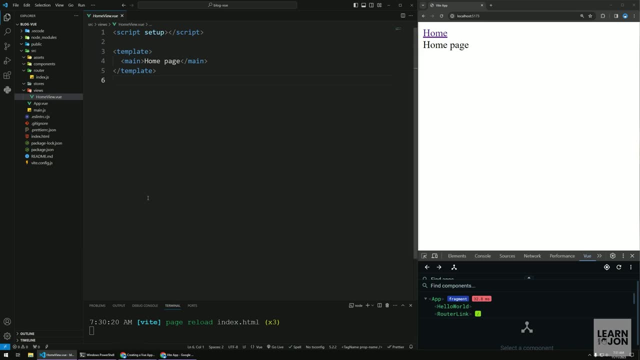 zinho. we're only going to have to go through the essentials as much as i can, and then we will go a bit deeper to single file components and actually building our website. in my previous video, which is the options api, i go in more details into the essentials and talking about all of this in more. 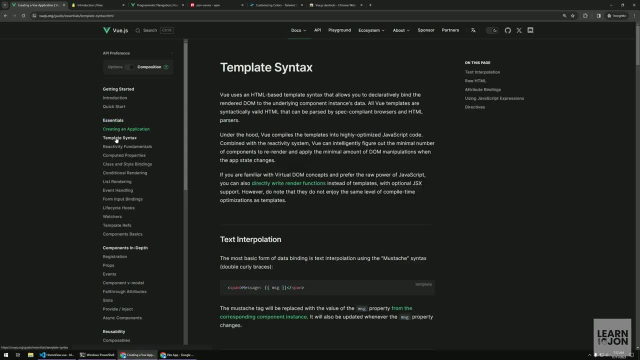 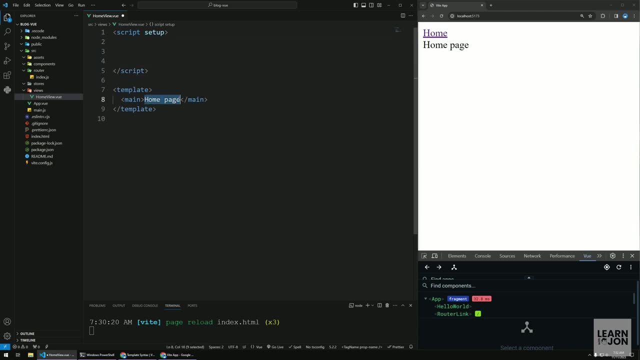 detail, which is kind of simpler because we're not using a built tool, so we are starting from scratch, so it looks much simpler and cleaner. anyway, let's get started by the template syntax. so the first home page here, just as a text, right, we want to show this as a dynamic data so i can create a 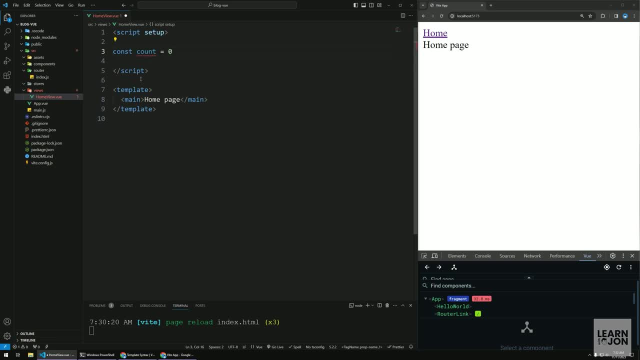 variable here. let's call it count and let's set it to zero. all right, so it says: right, here we are not using this count anywhere. so if down here i just say count, this will not change anything, because again, i am hard coding that text. but if i wrap it with two curly brackets and save it, you can see. 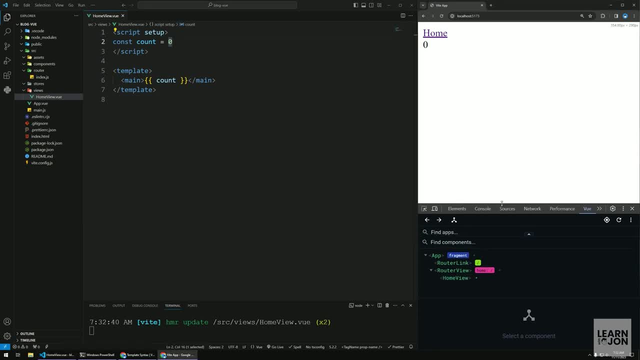 now i'm getting the value of that count variable and if we come down here inspect our home view, this view dev tools. by the way, i just want to say it's not, as it's not the best, i would say, because most of the time it breaks and you have to refresh. you can see it's not showing my data. 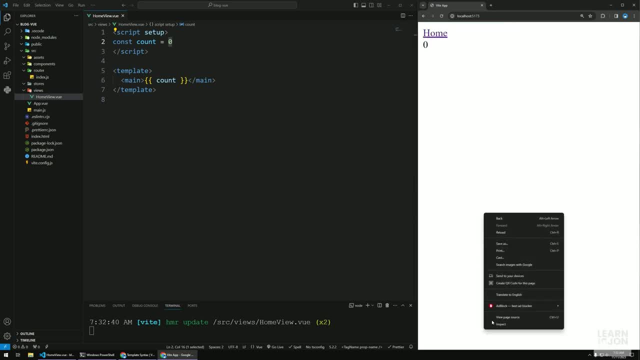 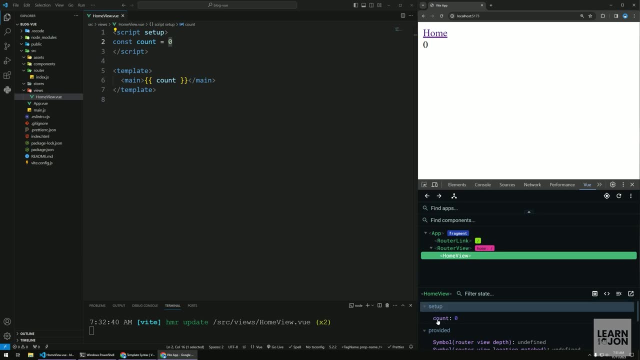 it should show the data down here. so let's close it, let's inspect it again, go to view, and there we go. now we have our setup function that has the count to zero. okay, so sometimes you have to do this with view dev tools anyway. so that's basically showing dynamic data on the 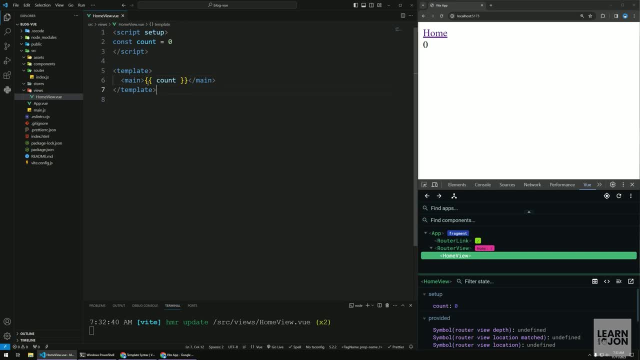 screen using this mustache syntax. now let's say i want to dynamically increase this number zero by clicking on a button, so let's change this main to a button, so like, just like that, and then pass that zero- or i'm sorry that count- into this button and let's just say number. 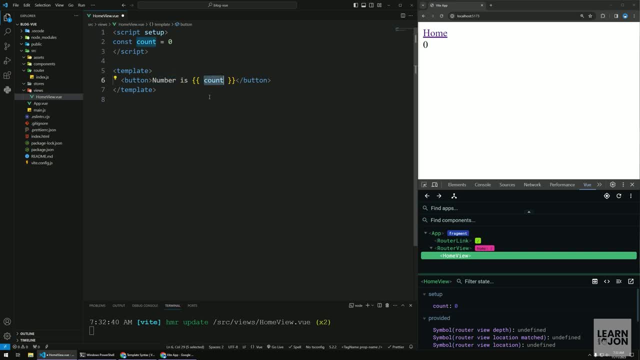 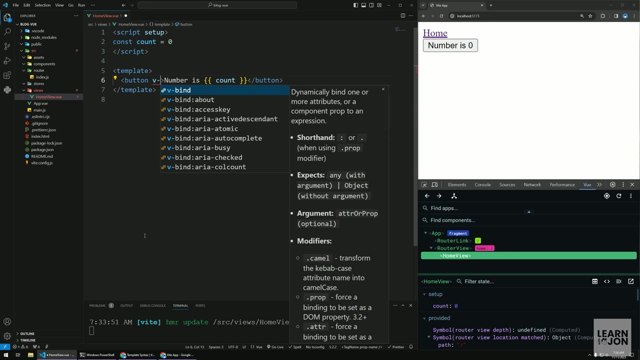 is. so this is a text and this is the dynamic data and we get the button up there. so now i want to click on this one, like basically saying unclick, kind of thing. but in view we have directives to do these things. so all the view directives start with v, dash and. 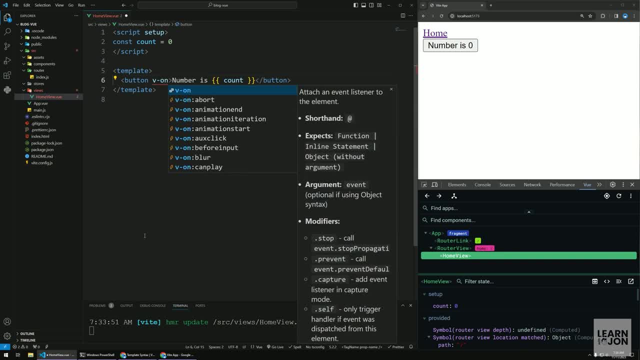 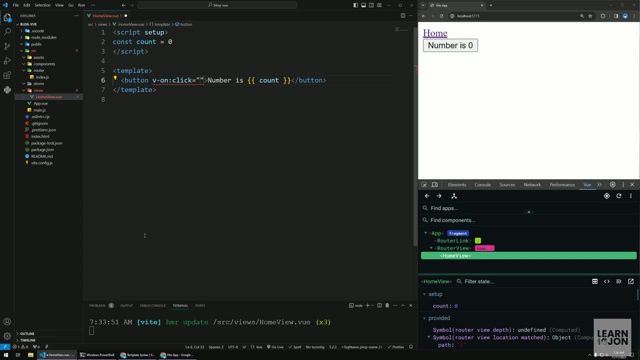 we have, for example, v on which lessons for a listener, for an event listener, and we have a colon and we can say: i want a lesson for a click, and what's going to happen when i click on this one? i want to increment that count. now you notice, here this count is already a dynamic. 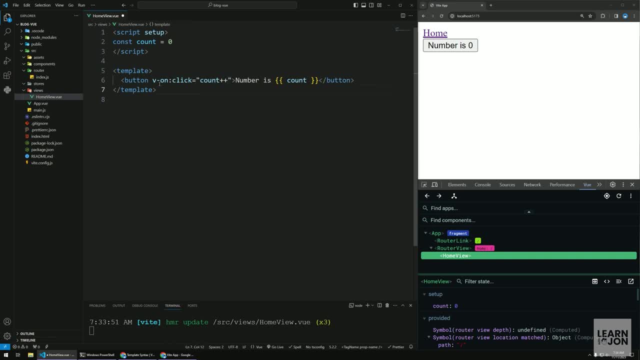 data, even though it's within this double quotes, because when we use the directives view, all the already knows this is going to be a dynamic data. It's not just a text anymore, So this would not work actually. So if I save it and press this button, nothing is changing on the DOM. But if 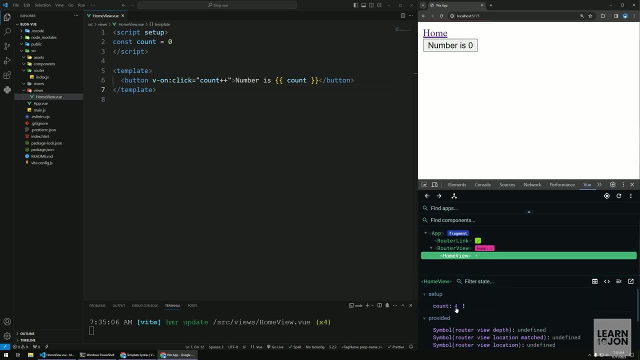 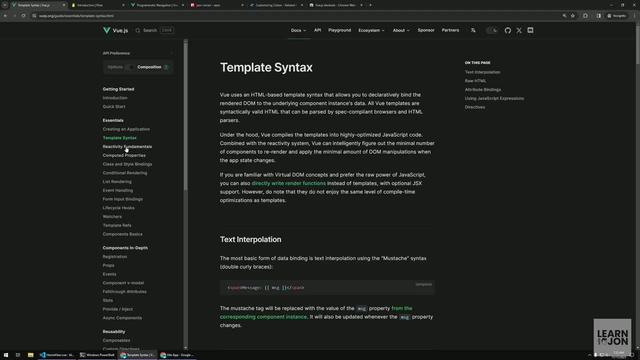 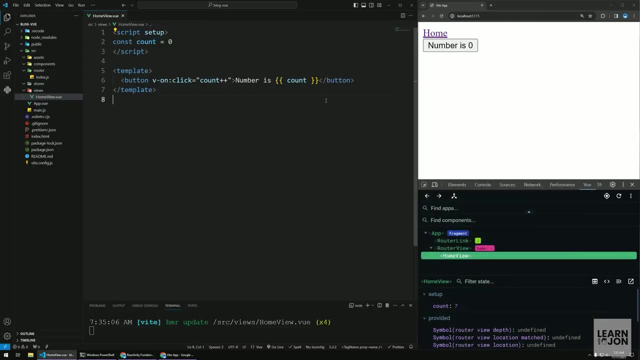 we refresh this countdown. here you can see it's actually working in the backend, but it's not shown on the screen. This is because this item is not reactive- Basically a reactive data. here we can read all about it. A reactive data is an alive data. if you will, It will change or update. 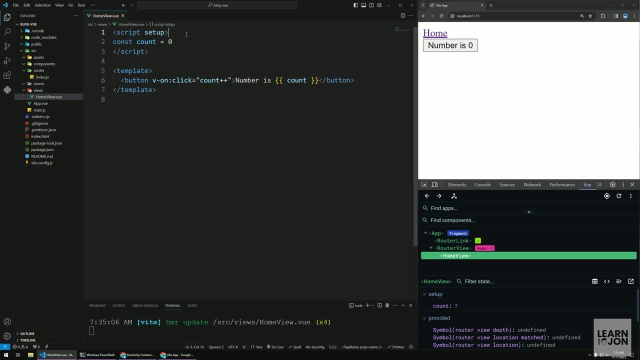 on the fly as we click on it. So with the script setup, in order to have reactive data, we need to import it from Vue, So we can say import ref, for example, from Vue, just like that. And now we need 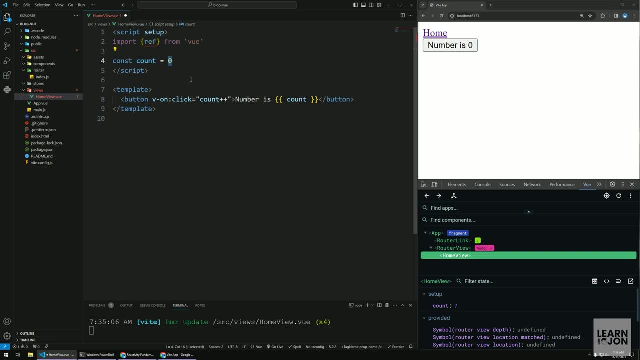 to wrap this zero in a ref, So we can use that ref, which is a function, and it accepts the initial value of this count. So we want to set the value of this count. So we want to set the value of this count. So we want to set. 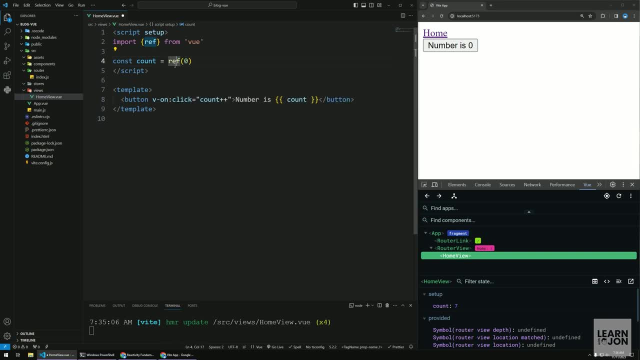 this count to zero. So we pass that zero as an argument to this ref method. Now, if I save this one and go to the home view, now you can see this one says ref in front of it or reactive. There is another way to make reactive data which I will show you in a second. So if I click on this one, 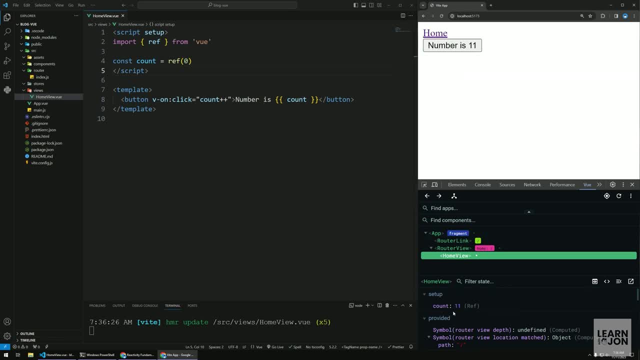 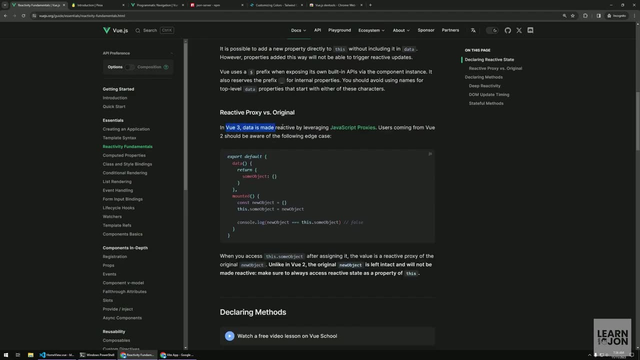 now you can see the number is increasing on the screen. This is because of that reactivity again, And if we read this page again in the options API in fact, you can see that Vuejs. it says Vue uses JavaScript proxies to make data reactive. 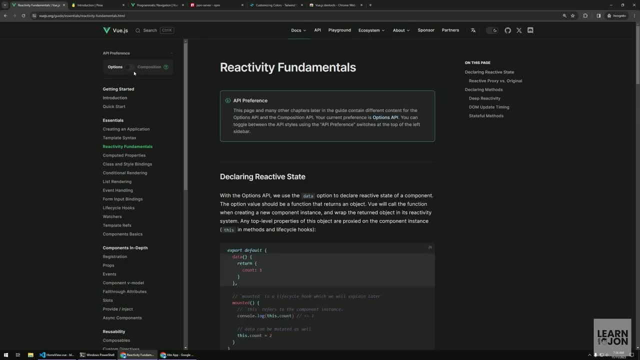 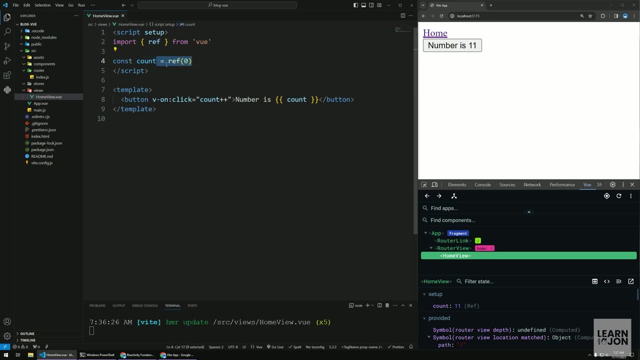 And again, we can read all about JavaScript proxies in here. So let's go back here and let's change this ref to another way of making reactive data. So ref is one common way to make reactive data, And then the other one is reactive. So that's just another way. I'm going to copy paste this one. 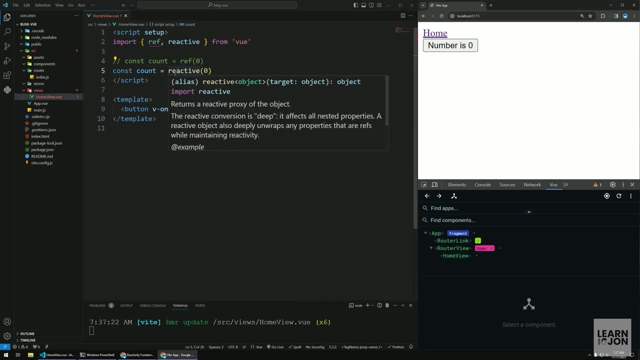 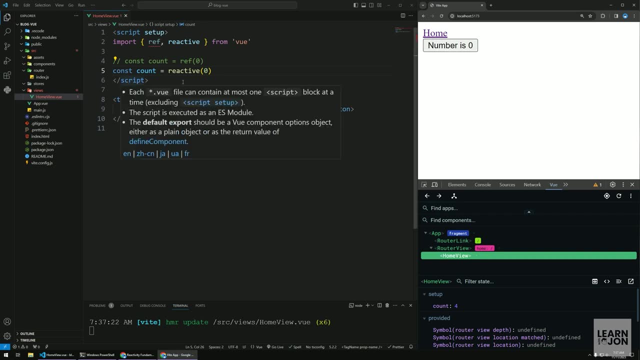 and comment this out and change this to reactive. So if I save this one and go to the home view again, you can see we have count, but it doesn't say anything in front of it, right? And if I click on this one, nothing changes. This is because reactive. 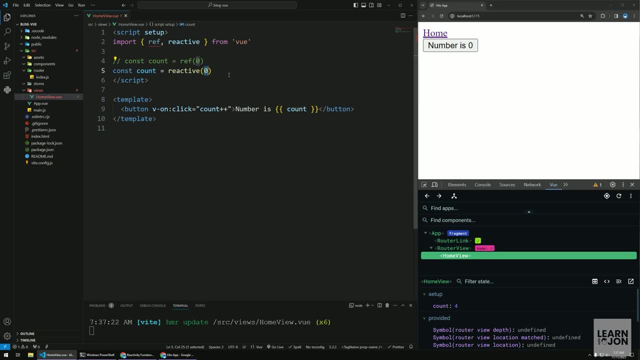 doesn't take a value, just like ref, This actually takes an object all the time. So we need to set the value of this count to zero. Now, right now, I'm calling this one count and this one count as well. This wouldn't work because this is kind of a wrapper. So if I call this state, for example: 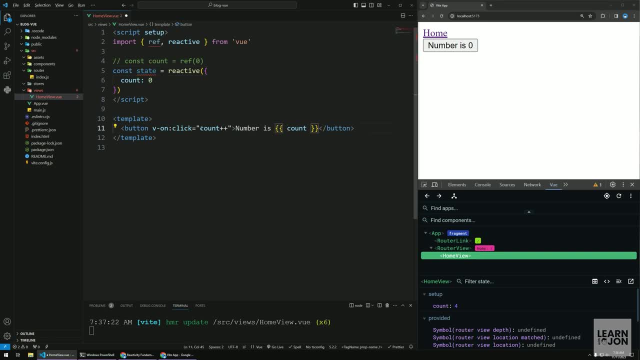 and now I have a count within the state. So in here I can just say statecount, just like that, And if I save this one, now go to the home view. Now we have a reactive state which has the count in it. So if I click on this one, 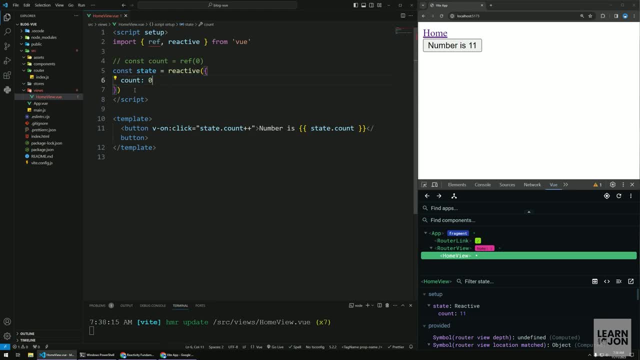 now it's working again. That is the first difference between ref and reactive: that ref can take the value of that variable as an argument, But with reactive we actually have to pass an object where the key is the value we want to use And the value is the initial value. 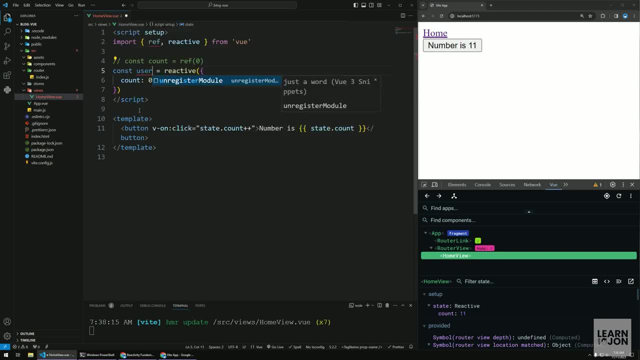 This is the best way when you have, for example, a user, and a user has many properties Like name, last name and so on. So we will use reactive and ref, both of them- in this project. Now, another difference between ref and reactive is how we call them within the script. So, if I 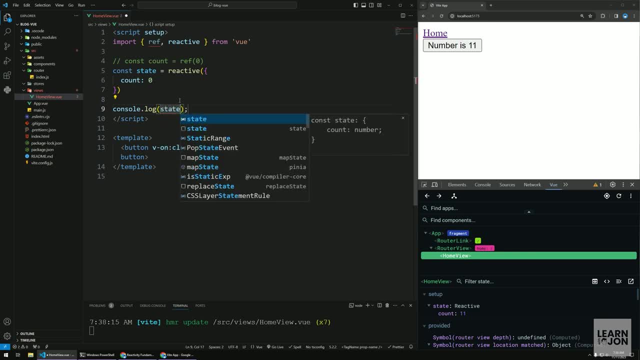 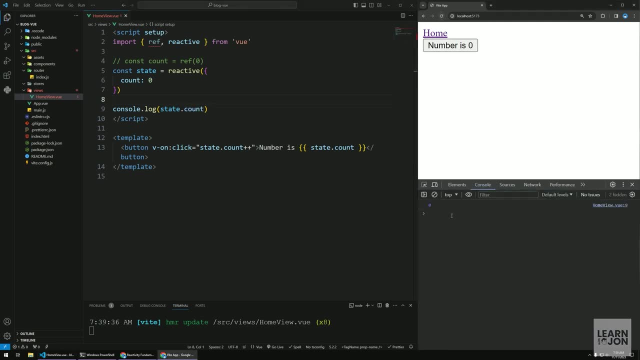 want to consolelog this count. I can just say statecount, just like calling an object right Statecount. So if I save this one and come to the console here and refresh this one So you can see I have zero here and I can't increment it here because this is not react. But we are getting what? 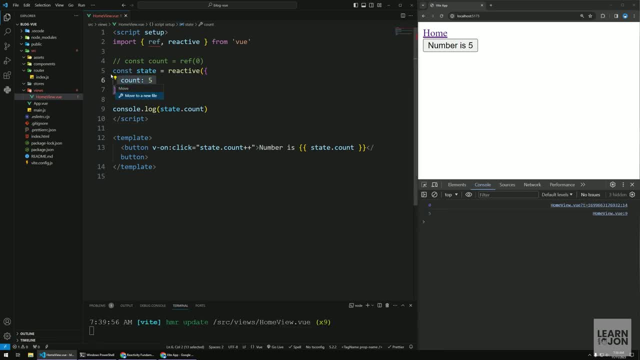 I want. So if I change this to five, of course I'm getting five. However, with ref I can't do that, So let me comment this out and bring this one back. So I want to get that count zero right. So 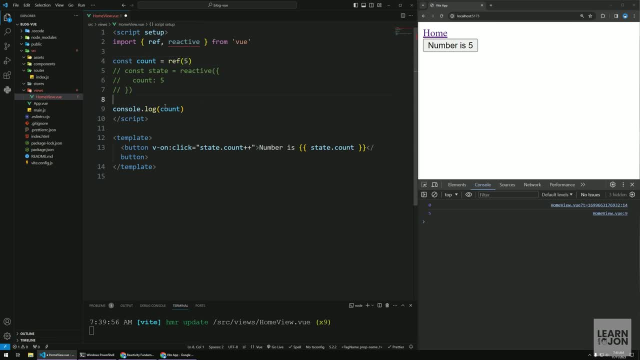 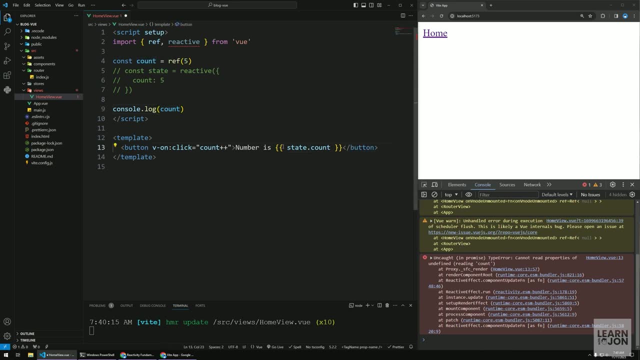 let's change it to five. So I want to get the value of five for this count. I can't just say consolelog count. You can see it's giving me. okay, sorry, this is actually the error from here, So I'm going to delete this one. All right, So refresh Right now. you can see it's not giving. 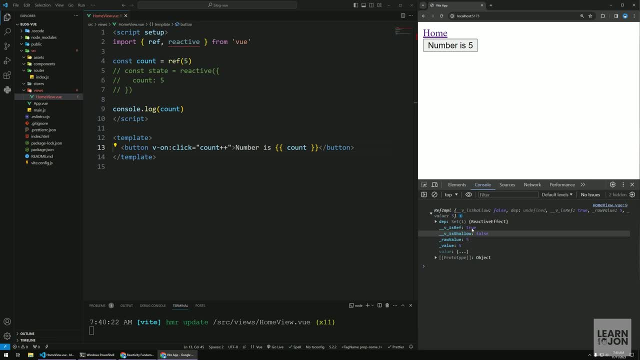 me number five. It's giving me an object with all these values and all these properties. The number thing is still works, because in here we don't have a problem. This is the problem here. So this ref doesn't give us the value of the count. We need to actually reach for the value by adding. 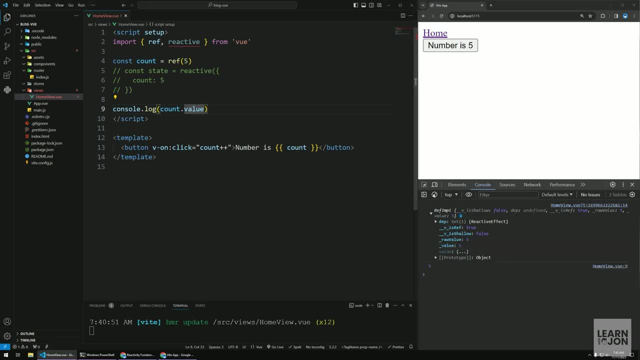 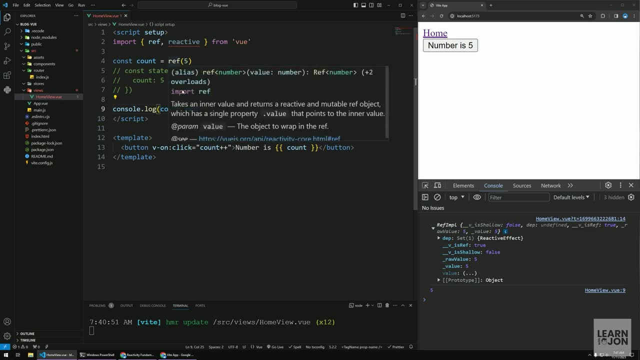 the value property And you can see it's down here. So if I save this one now, I'm getting number five. So this is again another difference between ref and reactive. If you want to reach the value of a ref within the script, you need to actually use the value property Within the markup. we don't. 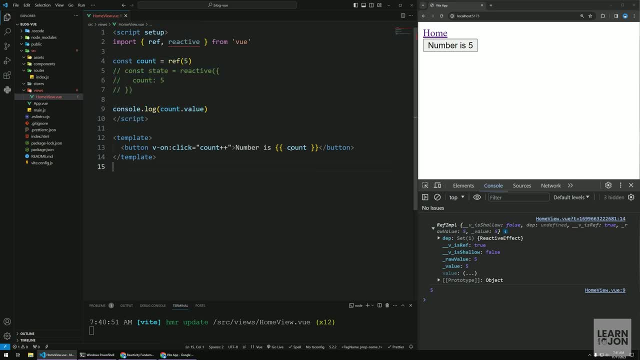 have to say countvalue. All right. So that's the difference between ref and reactive, And again we will use both of them in this course. For now I'm going to keep the ref up there And let's talk about some of the view directives. So view directives are very useful to add dynamic data. 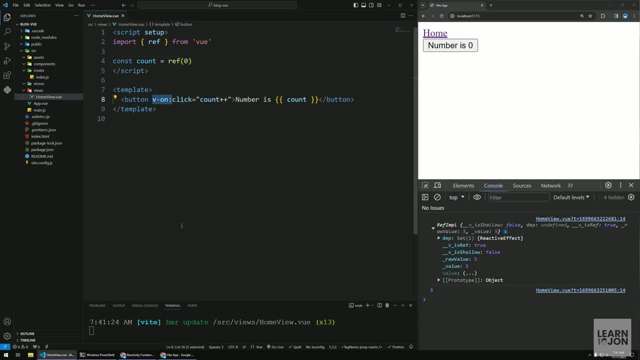 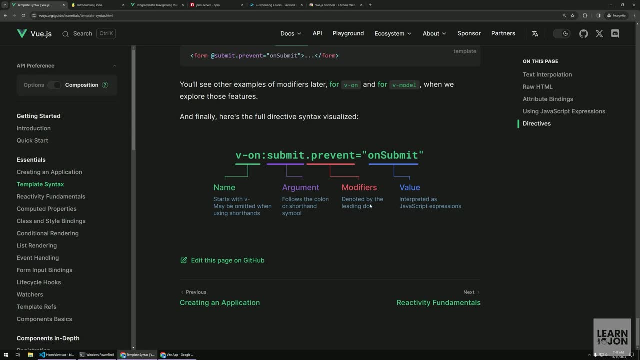 to our HTMLs, Just like here. we saw V on, And I'm going to go back to the view documentation and go down all the way here and look at this image. Basically, this is a text that goes on an HTML element. I'm going to close this terminal too. Don't need it, So you. 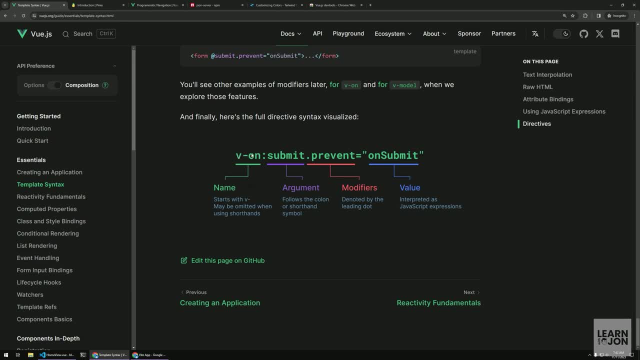 can see, we have a directive name that starts with V, dash, And sometimes it can be omitted if there is a shorthand, And we will see the shorthands in a second, And then we have a colon And then the argument, whatever we want to pass into. Sometimes it's an event, listener, if it's V on. 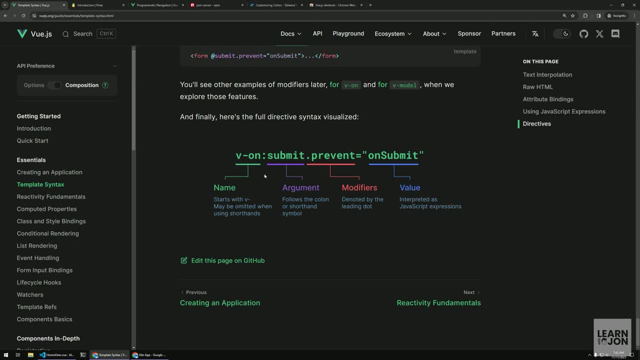 Sometimes it's an HTML attribute, if it's V bind, for example, And then we have modifiers So we can say, for example, dot something, That is the modifier- And prevent. It's the same thing to say, for example, prevent the default Once. for example, we have dot once. 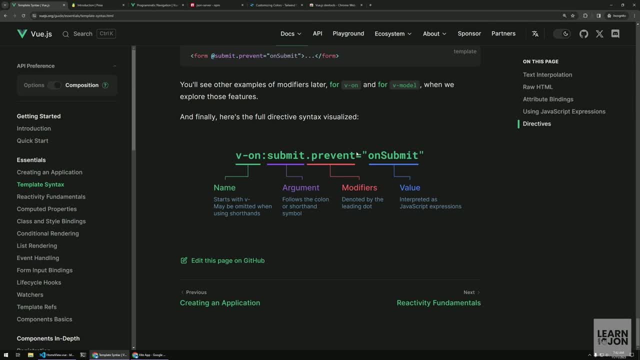 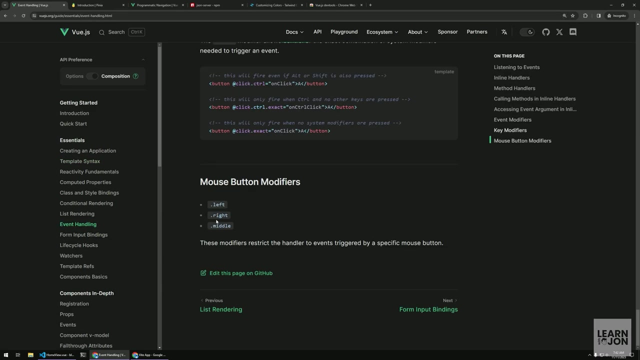 That will run that event only one time. And then on the other side of this expression of course, we have a JavaScript expression. So whatever is going to happen here when we click or submit or watch or whatever, So if we go to event handling here we can see all the- if I can find it. 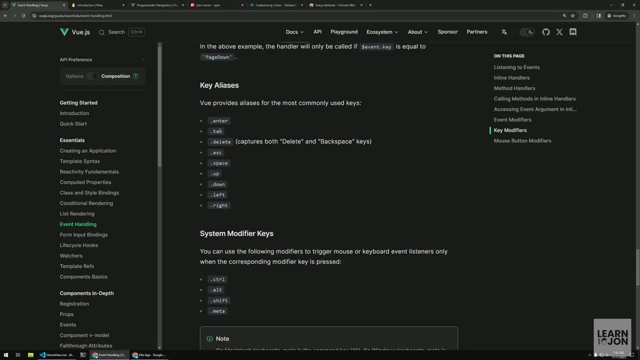 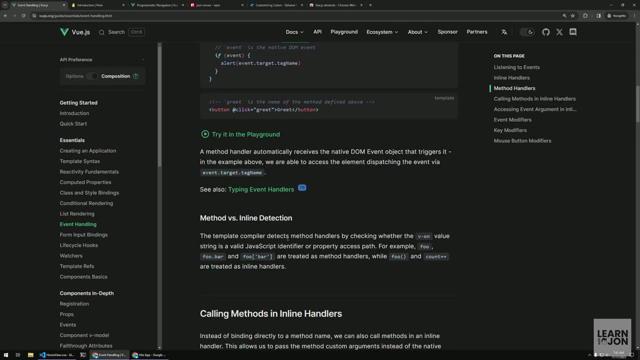 you see, we have key aliases Like we can lesson for enter. These are the common ones. That's why they list it out here. We have modifiers like stop, prevent, self-capture and so on, And all the other listeners from JavaScript. So let's talk about some of them Again. in my previous 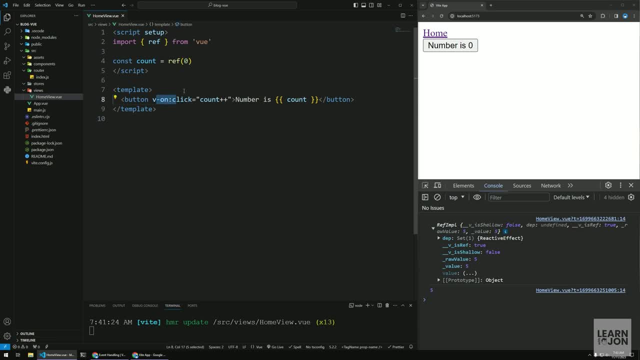 video we go over the view directives in more depth, But here I'm just going to mention the most common ones. So of course we have V on And the shorthand for V on- because it's quite often- is just an at. So if we say at click, it's the same thing to say V on click. So another one is V bind. 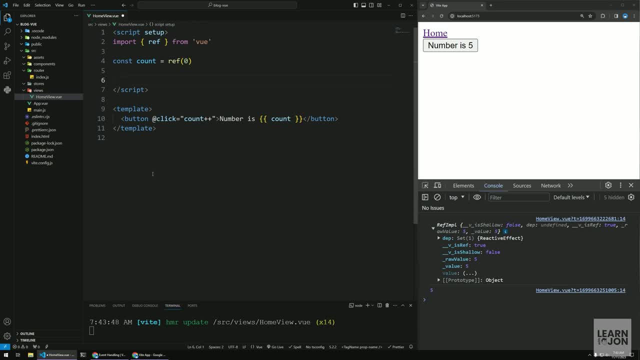 And that will bind an attribute To a dynamic data. So let's say I have a variable here that says my class And I'm going to set it to my class. So I don't have this CSS class, for example, But I want to bind my CSS class down. 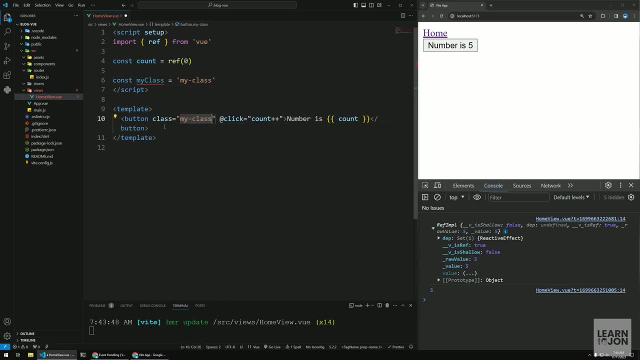 here And normally I say my class just like that. So I'm passing my class text up here And I can just add a style tag down here and say, for example, my class give it a color of blue. So 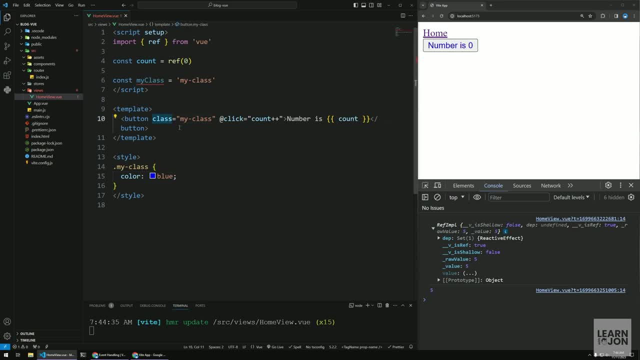 the text will be blue. Now this is working and it's fine. I want to pass this one as a dynamic data rather than just pass hard coding it, Because if I change this one up here, nothing changes, Because why would it? It's not bound, So we can do so by V. 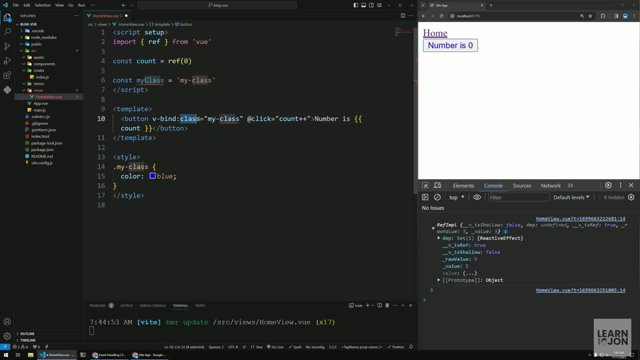 bind And again colon. So V bind binds this class to this one And you can see it's giving me error because this my class is not the right way to call it. So we don't have this my class And this syntax is not correct. So we need to pass that my class up there. 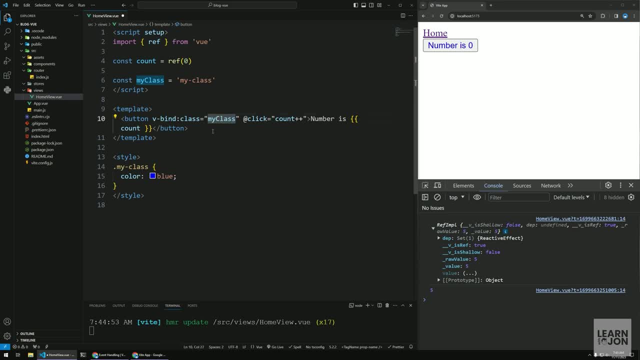 So this variable reference to this V bind as a dynamic data. if I save this, we still get the blue, because now we are calling this one And if we inspect the element you can see it has my class, my dash class. So this is very nice. First of all, V bind is quite often just like the click or the 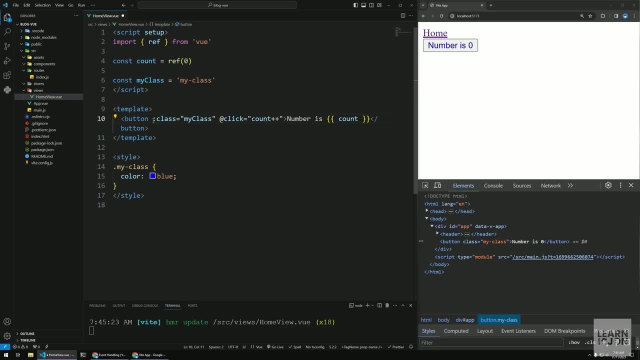 event listener. There is a shorthand and that is just a colon. So if I say colon class, that'll work the same. Now here, remember, we said we can pass any JavaScript expression, For example, apply conditional classes. So I can say, for example, if it is true, if my condition is true, 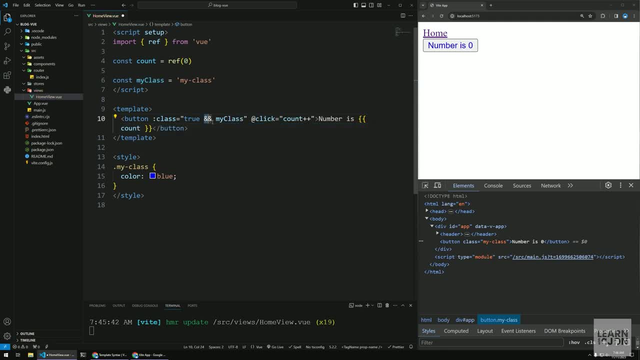 apply that my class, And I'm using logical and here. So if this condition is true, this will be applied. Otherwise, nothing will happen. So right now I'm saying true. If it's true, apply to my class. apply this, my class. Okay, And that's why the text is blue. If I change this to: 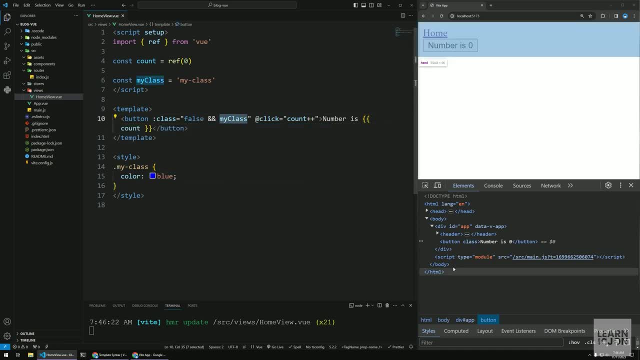 false, of course, nothing is going to be applied. So this is completely ignored And you can see I have nothing on my button. no class. We have other directives, like V if and V show and other things, which we will cover as we build our. 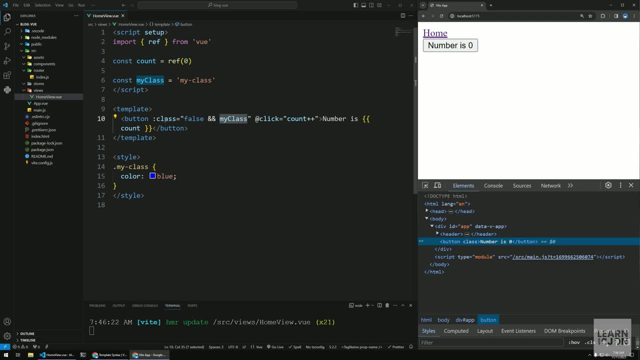 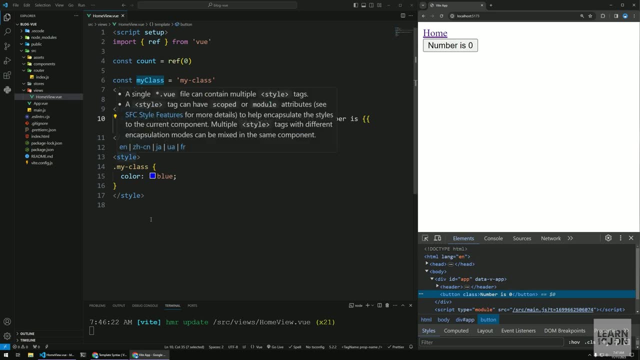 application. So I don't want to waste your time and, you know, go over them and then use them again in the application. So when we get to them, while we are building our application, I can explain all those directives. All right, So before we get into building our application, I just want 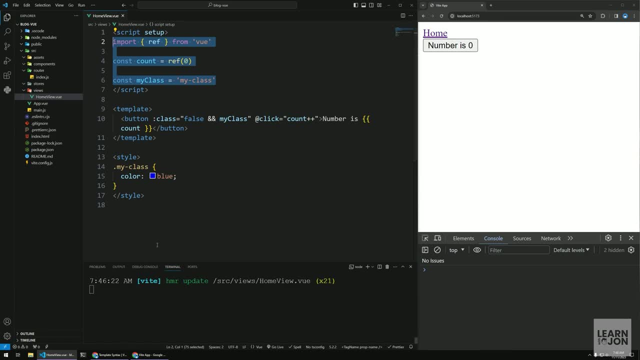 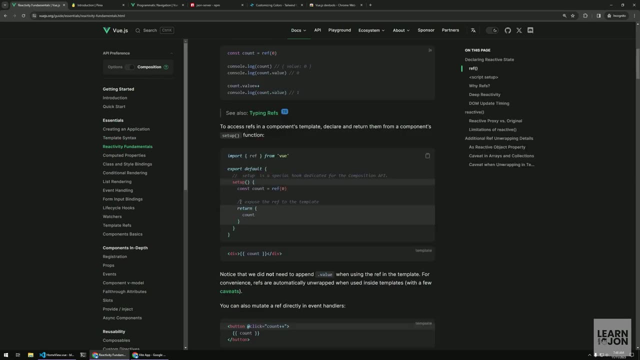 to mention the difference between the script setup and the setup function. So Vuejs offers two APIs, options and composition. And within the composition API, we have two syntax. One is the script setup, which we are using, One is the setup function. 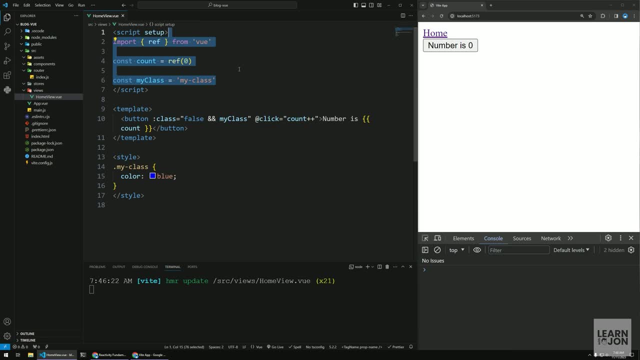 And I just want to briefly show you what's the difference and how crazy it is. So I'm going to cut all of this out for a second. And we need to have that export default. And now this is an object right. This is kind of like a component, And within this component we will have all sorts. 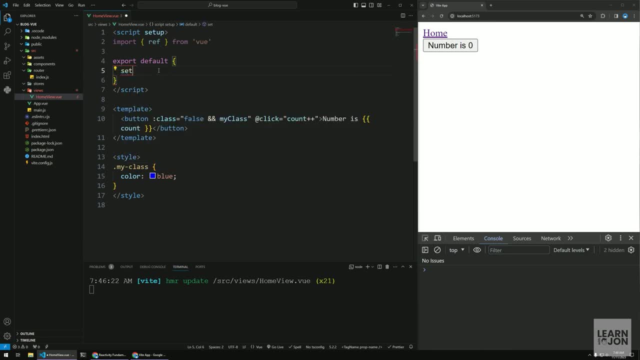 of data, So one of them is setup. This is the most important one, So these are called options And this setup function returns a value. Now you can see, this is giving me all sorts of error, because it says you cannot have this setup syntax up there if you are using setup function. So I 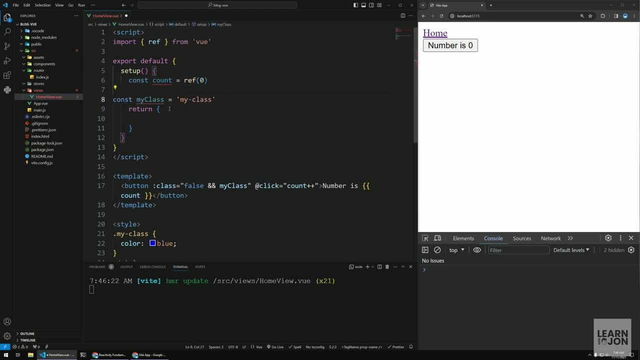 can delete that one. I can paste that code that I had before. So two variables, We have a ref and we have my class. Now this would not work down here. If I save it, you can see warning: nothing is working because we actually need to return whatever we use in our setup function. 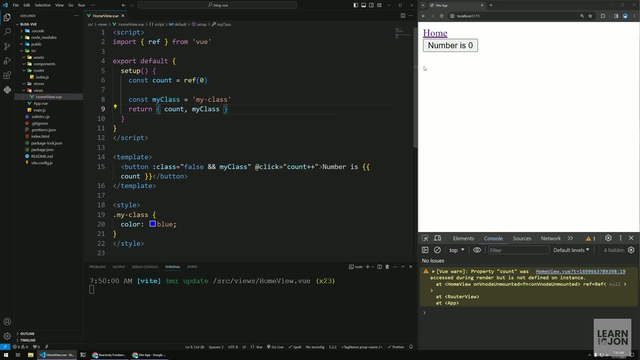 So we have to specifically return those values that we want to use. If I save this one now, it's working fine, But you can see before it was just two line of code. Now I have to use the export default, I have to use the setup And later on, when we have our 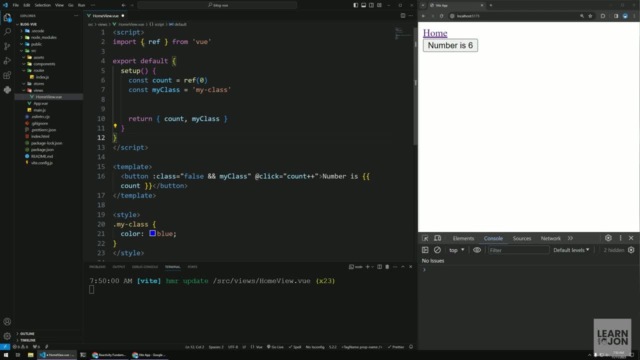 components, it becomes even more evident that the script setup is much, much easier because you have to import everything with the setup function And then you have to specifically tell the setup function that I am using these stuff. And again, when we get to the components, 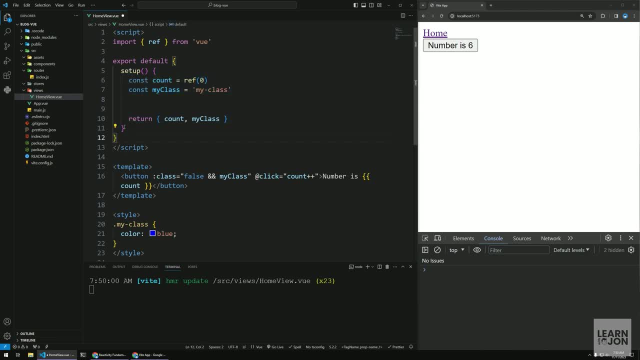 I will come back here and show you an example of a script setup and the setup function. Let's turn this back to the way it was And I'm going to delete actually everything because I don't need it, But I'm going to put the setup up here And I'm going to delete this one too. 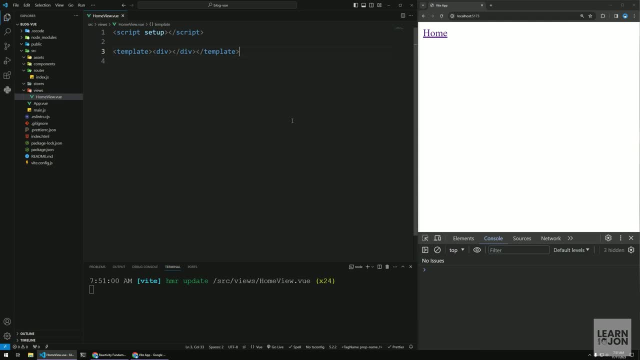 And this one. So we're going to start building our application And I'm going to bring some HTML CSS code here, But before that, because I'm using Sass in my CSS, I'm going to install Sass or SCSS. So we can do so by saying: npm install-d sass. Alrighty, so I can run the local. 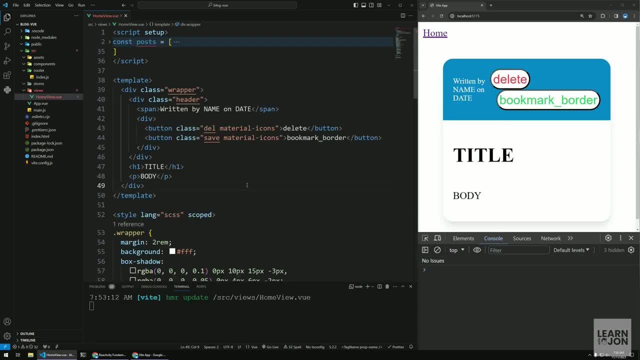 server again. So let me grab The markup. Okay, so I pasted some code here, which I will explain in a second, But before we do that, I'm going to paste some CSS for the whole application. So let's create a file within the assets. 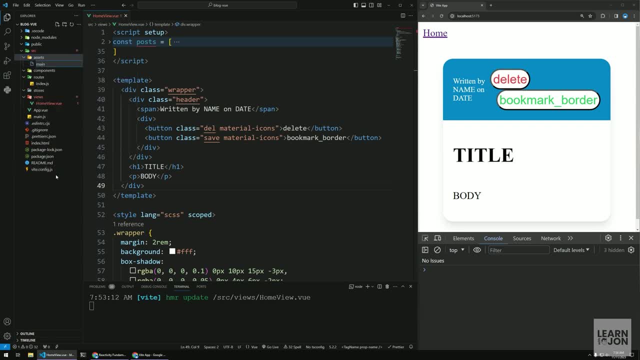 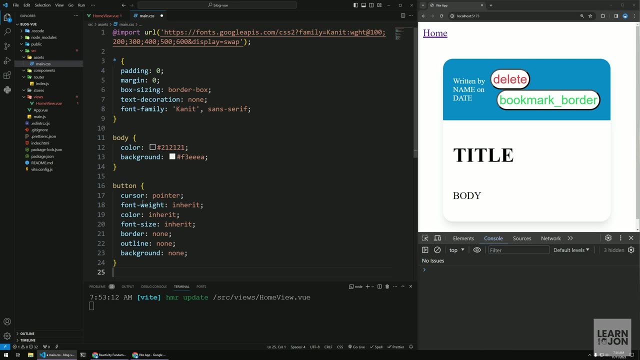 folder. So let's create a CSS file and I'm going to call it maincss And I'm just going to paste some code here. So I have a Google font bringing in and resetting my CSS, just some colors and some stuff. So we need to save this one Now within our mainjs. we actually have to tell the application that we are. 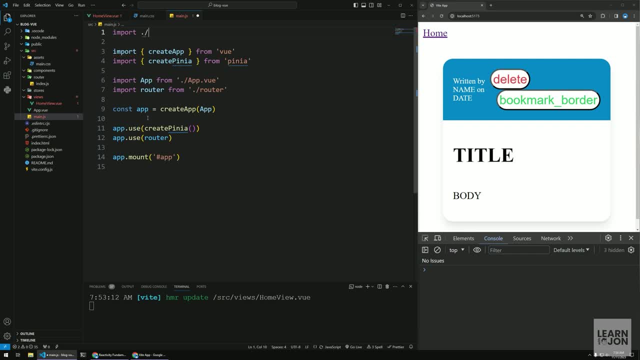 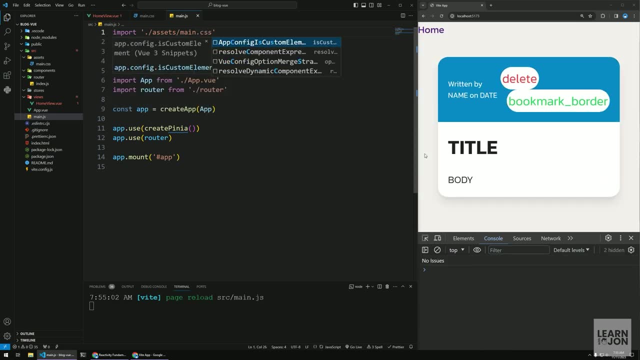 using that CSS And we can do so just by importing it, So I can say it's within the assets and I called it maincss. So if I save it, you can see the font is applied And let's go back to that markup that I have, which again. 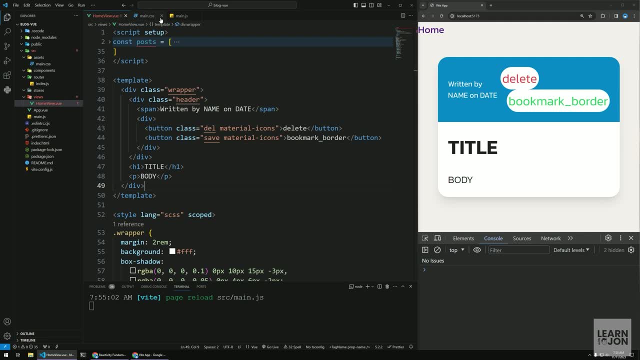 all of this code will be available in a GitHub repo, So I'm going to delete the maincss and mainjs. Let me explain what's happening here. So I have a markup, which is basically this box right here which will contain the posts which we are going to show, Just some text and some code. So I'm going to paste some code here. 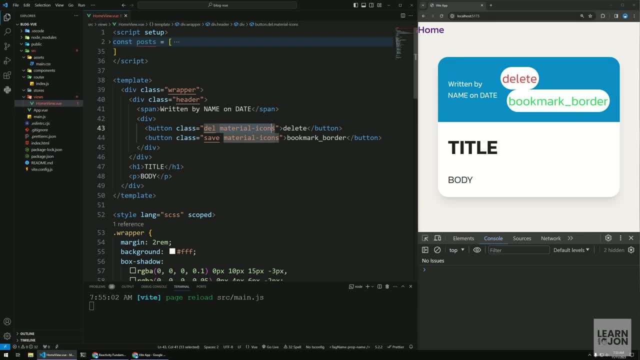 So I'm going to paste some code here. So I have a markup which is basically this box right here which will contain the posts which we are going to show, just some text and some icons. For the icons I'm using material icons which I haven't linked it yet, So let's do that first. 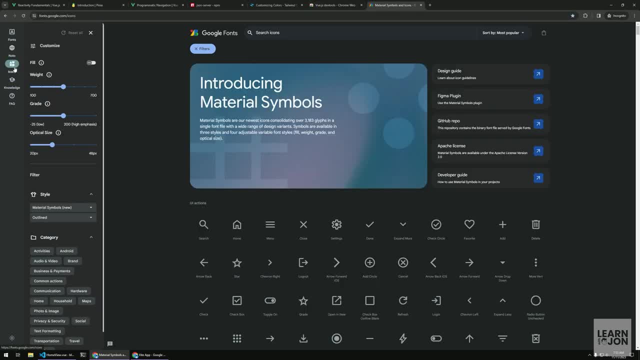 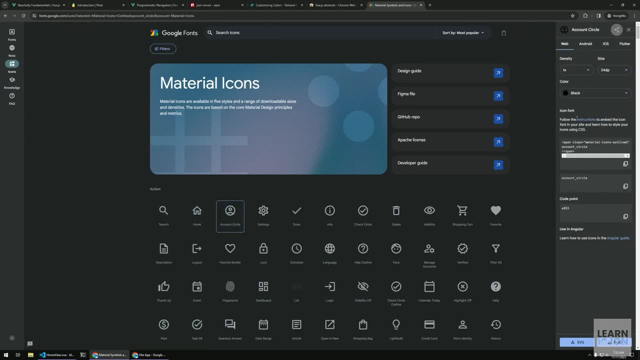 You can go to Google Fonts and go to the icons on the left side and choose the material icons, not the symbols, And if we select any icon and go to the instruction on the right hand side here, this will give us that link we need. 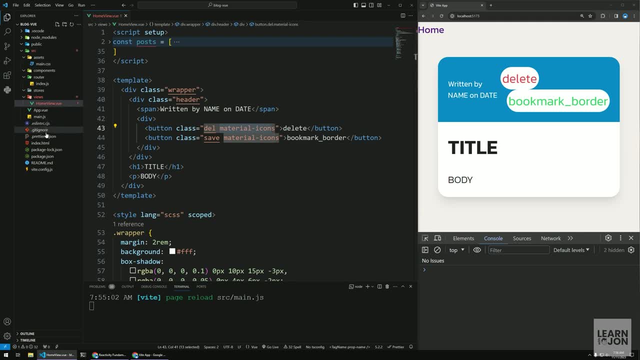 So I'm going to copy this one. Let's go back to the project in the indexhtml. We are going to paste this on the head in the head. sorry, not on the head in the head. Sorry, not on the head in the head in the head. 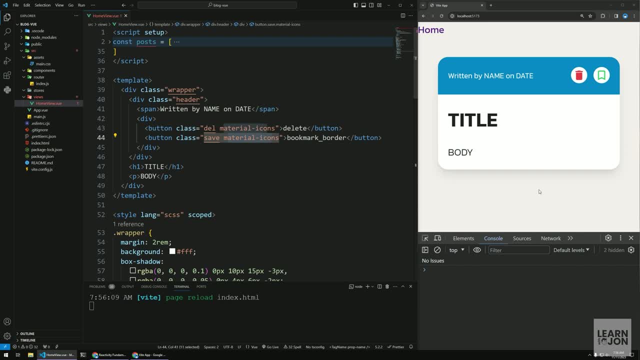 save it. now we get the icons, and these are all really just css and html. nothing fancy here, but anyway, let me explain what's going on. so we have a header with two buttons- delete and save- where the user can delete or save a post, and then it says when and who posted this, and then the body. 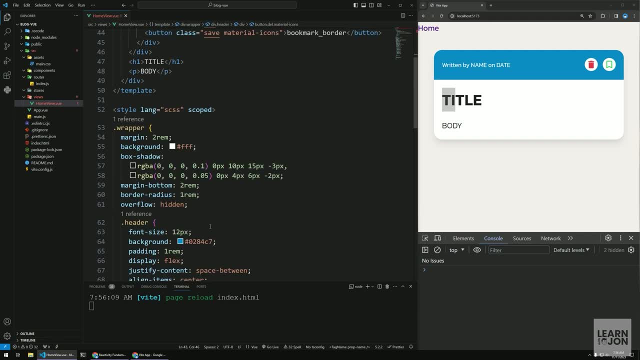 of the post. within my style tag, you can see i have few extra things added. first, is this lang attribute that specifies that this style is actually sass, or i am using a pre-processor, basically, so you might have seen this in other languages, but i'm specifying that i'm using sass. 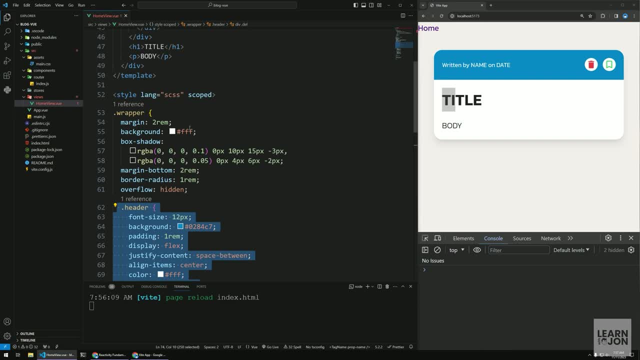 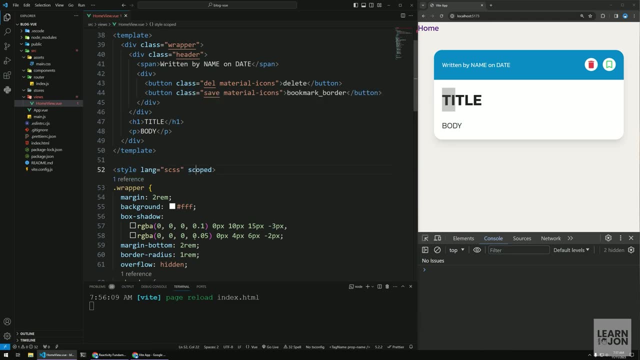 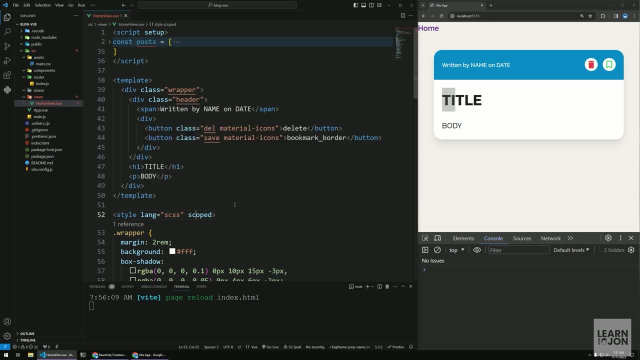 as my css, so i can nest these classes within each other. and also we have this scoped attribute. this might be new to you, but the scoped attribute, it will make this a style tag scoped to this component. and again, this is a beauty of vuejs and a single file component that everything can. 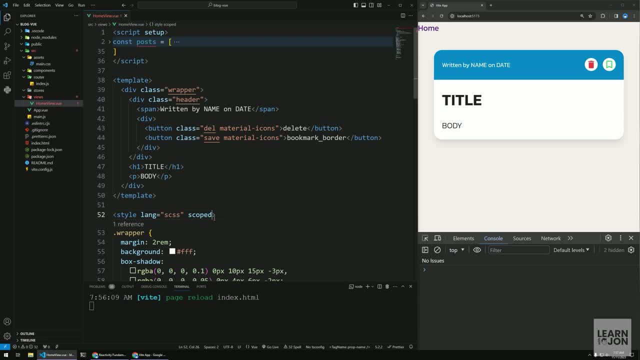 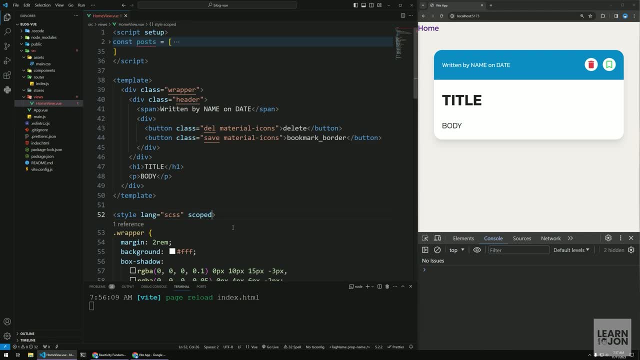 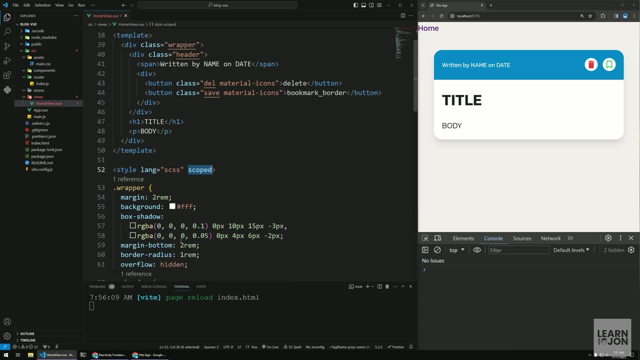 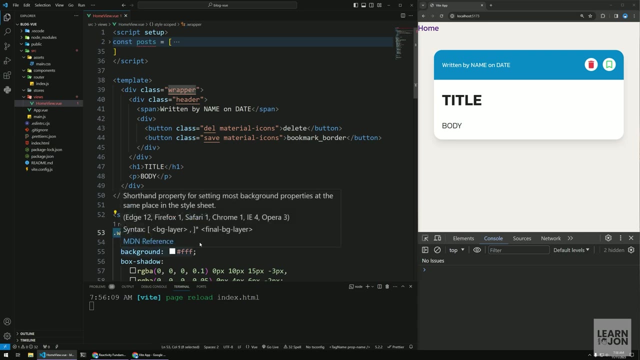 our job a lot easier and it follows the separation of concern concept. so basically, again, this scoped variable, if we add it to our style tag, it makes sure it will make sure this, these styles, stay in this component. so if we have another wrapper outside of this component, 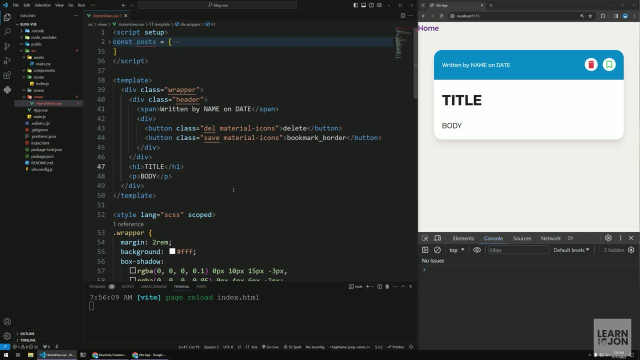 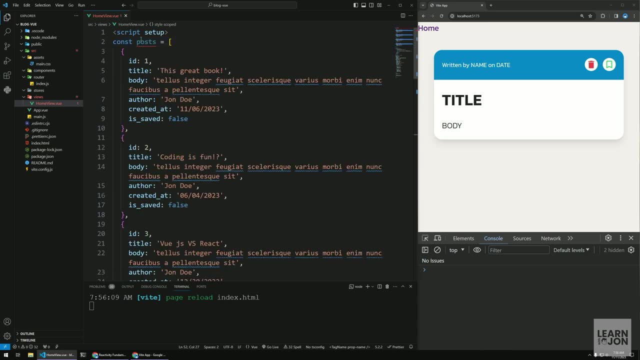 with the same class, this will not interfere with that one. so that's just basically the style scoped. now within my script, i also pasted an array of posts, so these are just hard-coded posts. there's nothing fancy here. and within each object which is a post, 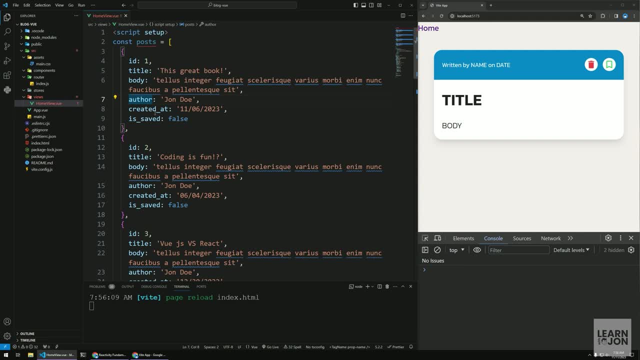 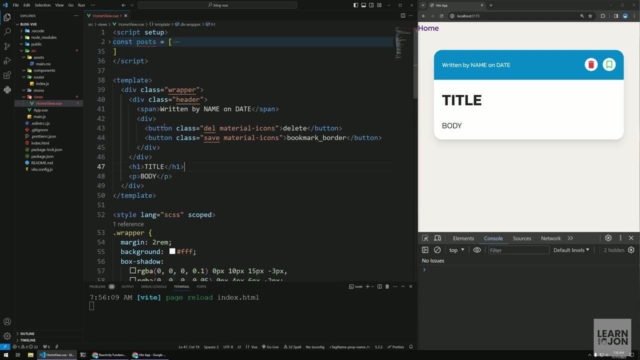 i have an id, title, body, author, so the author of the page, and the created app property, which is date, and is it saved or not, which by default is false. now, what i want to do: i want to show these on the screen and for each post which i have- four- i want to show a card. so let's do this. 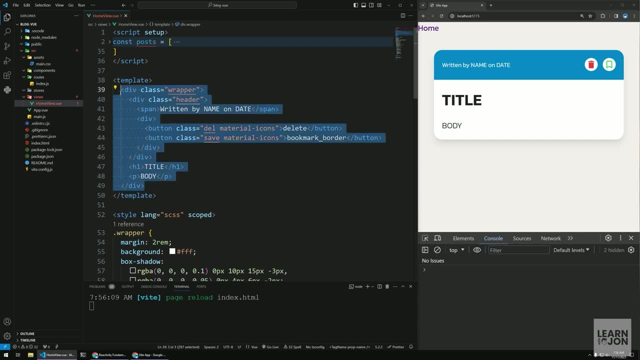 so i can wrap this whole thing within a div, so i can just say div. and now, on this wrapper, i want to repeat this whole thing here. we know, for example, to loop over an array we would use a for in loop or for each loop or something like that in javascript, but within 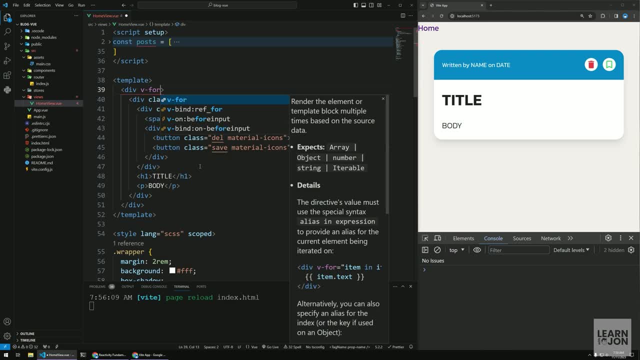 the template of a vjs. we have a directive called v4 and, as the name suggests, this is a v4 loop or for in loop. sorry, it's a for in loop in javascript. so we can say for every post in post just like: do something. now what do we want to do with this post? i want to change these hard-coded properties. 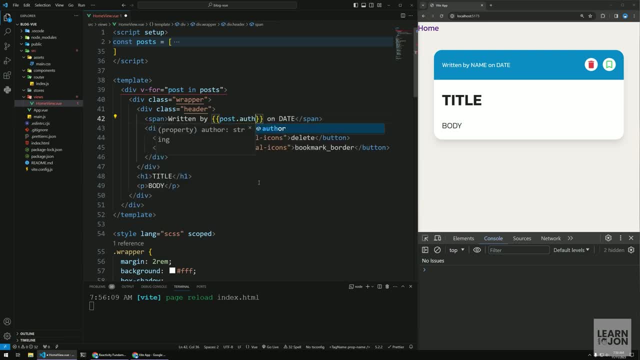 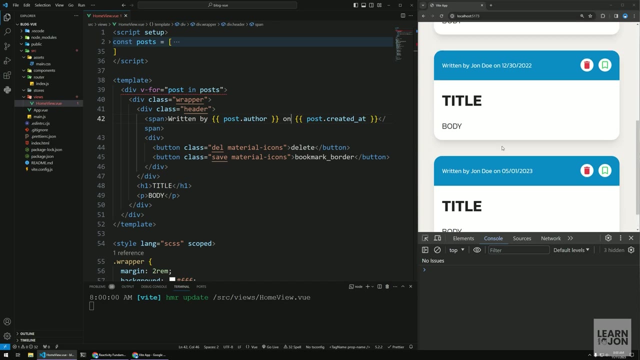 to dynamic properties. so post dot. author. i have that one for the date i can say post dot created at. and you notice i'm using the master syntax so if i save this one you can see i actually have four cards already and the names are pretty much the same. i can change one of them manually and 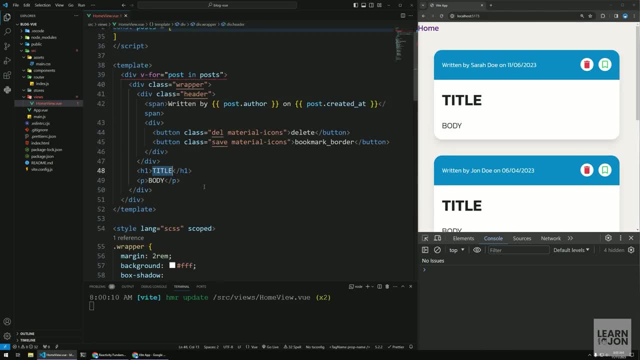 you can see now it says sarah anyway. so let's do the same thing here, and i'm going to change the same thing for body and the title. i'm going to select both of them and say post, dot, title, and then for this one i'm going to say body, awesome, done, finish. and you can see how easy it was. so i 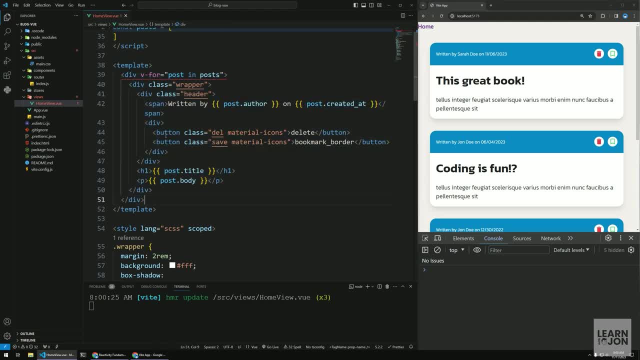 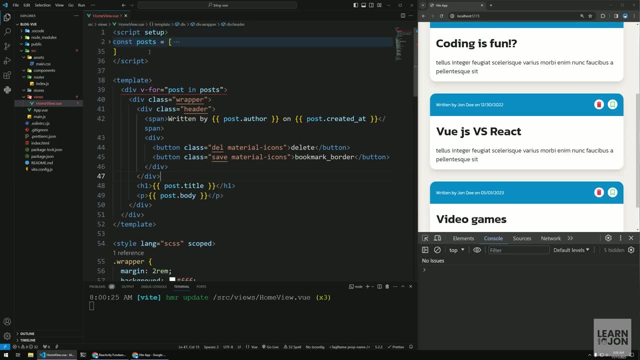 don't have to repeat myself like a normal html. i don't have to have four different divs, that repeating the same thing over and over again, so we can just loop over them and render for each item in our array. render a card. now you notice i'm getting this vaguely red red line here that says: 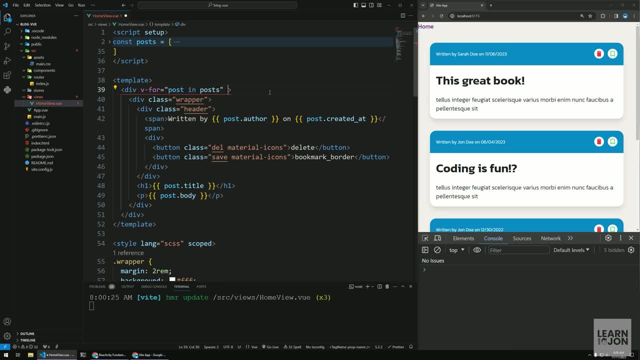 there's something wrong here now if you always recommend to provide a key and bind it to a specific unique value in your for loops and we can do so by binding the key, so we bind on the key attribute and then set it to the post id, because 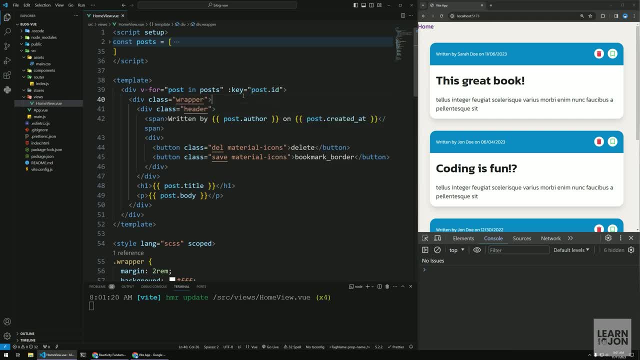 we know that post id is unique for all of them, so you can see that error is gone and the code is working just fine. this is a good place to make a component, because we are in the home view and we are hard coding this one, which is: 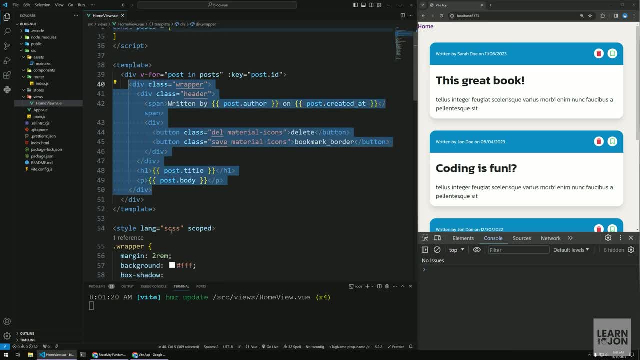 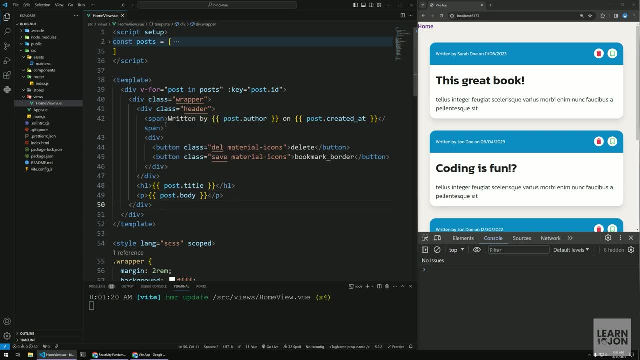 clearly as a card within the home view, so kind of it doesn't belong here. so we can separate this or we can extract this to its own component, and i'm going to grab this one because i want to use that wrapper for something else. so let's create a component within our components folder. i'm going 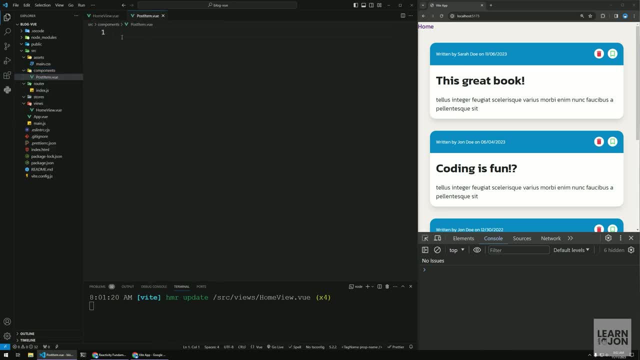 to create a new file and just call it post item dot. view. to get the boilerplate of a view component, we can say v, something like v base. so this is from that view snippet extension. so if i say v base and i have all these options, that gives me, so you can see here template. 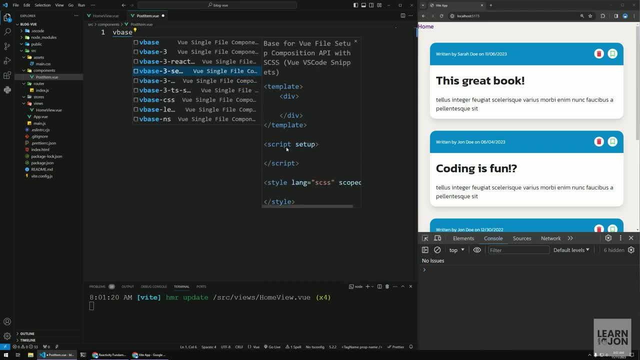 div script setup. yada yada, yada. and this one gives me a script setup. so view v base 3 setup. i can use it, but i i normally don't use it, i just hard. i just type everything myself. so i like the script tag on. 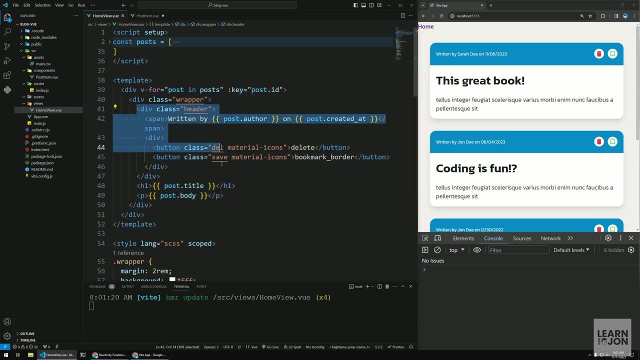 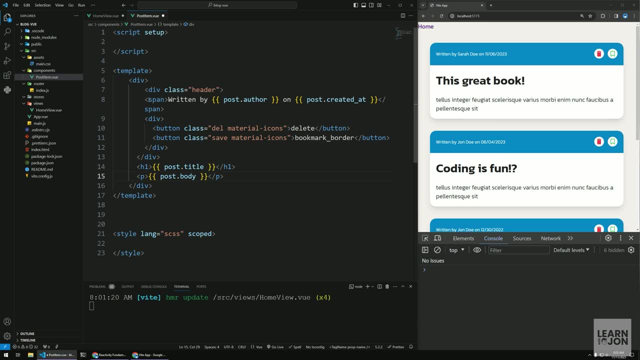 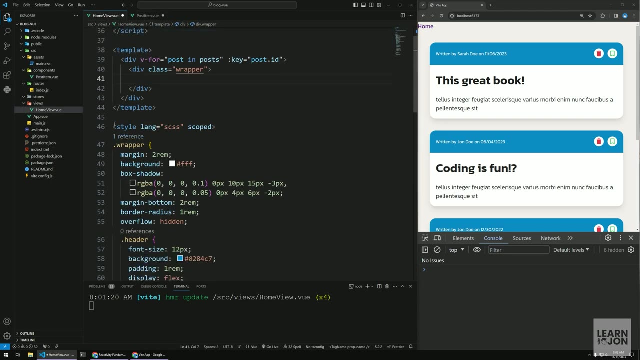 the top and now within this, we can bring this card. i'm going to grab everything here, okay, so i'm going to leave the wrapper and that v4 in here. so back to the item within this div i'm going to wrap. now this is our wrapper, so let's bring the styles too. i'm just going to copy everything, even though 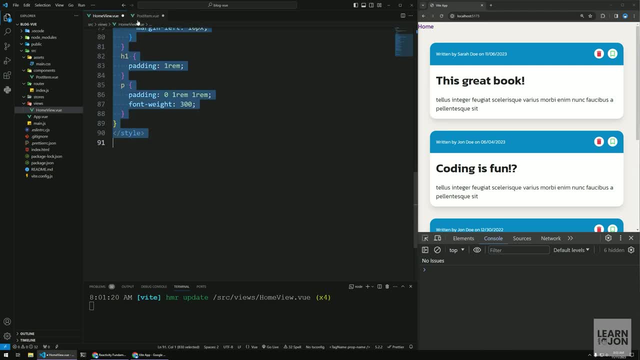 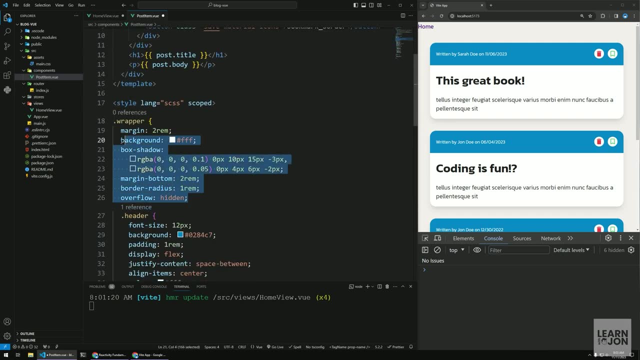 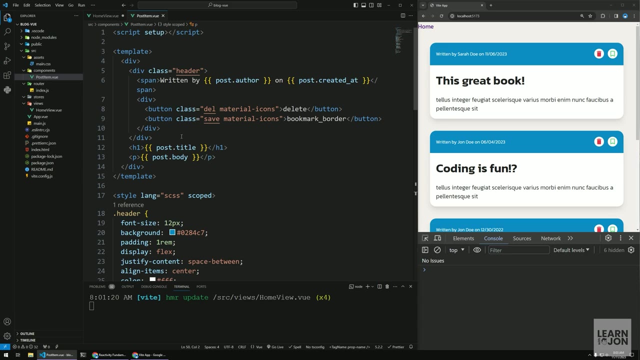 i don't need the wrapper, but i'm going to copy this, bring it back here, replace this style tag and go up there. delete the wrapper because i don't have it anymore. something wrong here because of this. okay, if i save this one, nothing changes, because we're not doing anything just yet in. 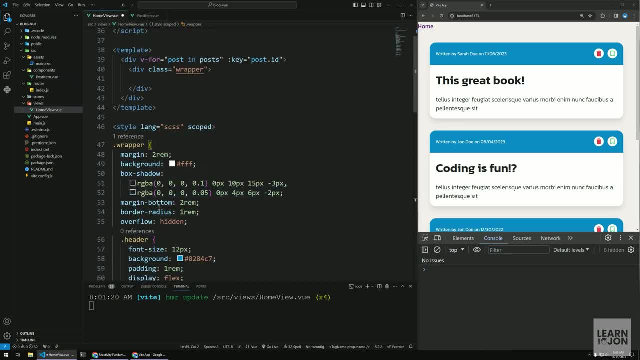 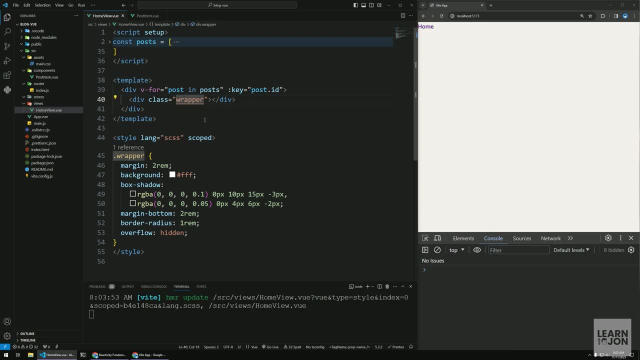 here i'm going to delete every style except the wrapper. so all the way to here and close that curly bracket. there we go, and now we actually need to import that one in here. so now we are using our external component. this is a good way to have an example. so first of all, let's bring 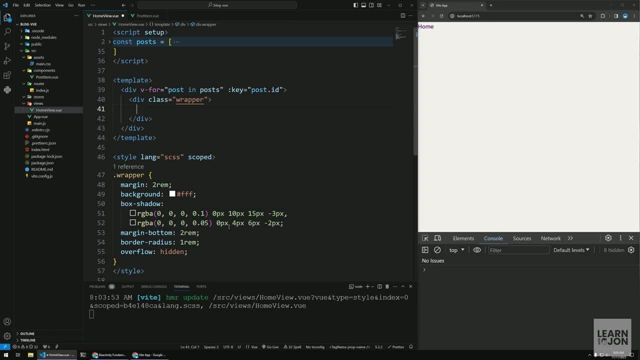 that one in and we can just use it as an html kind of like html element so we can say post item. now, sometimes vs code helps us to import it automatically. sometimes it doesn't, so we can try it up here, see if it works again. sometimes it works, sometimes it doesn't. so if i say post item, 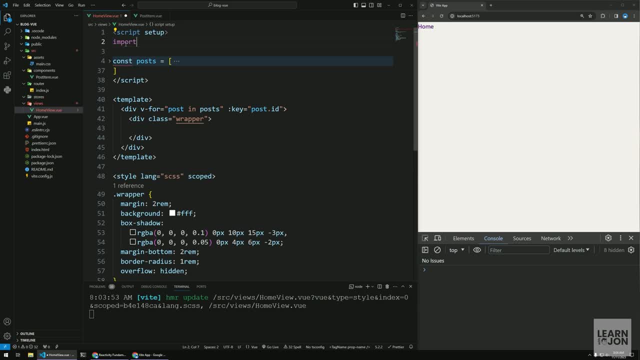 recognize it. for some reason sometimes works, sometimes it doesn't. so import post item. from now we can here use the at sign because remember in the vid config we said that at sign is an alias for our source folder. so we can just say at sign, that means the source folder, components and we 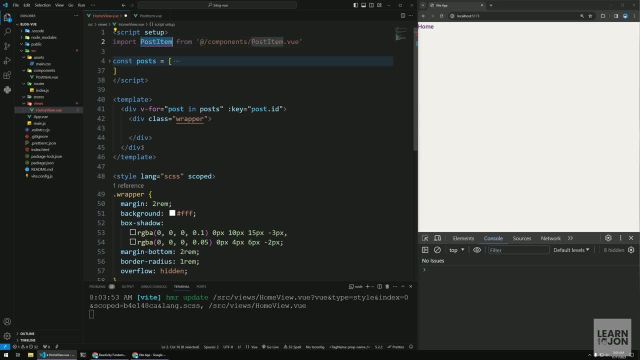 called it post item, that view. now i can use this within my template. i can say post item and close it like that, or i can just use a self-closing tag like that. so if i say post item and close it like this and if i save this one, we will get some errors. there we go, because we are trying to reach. 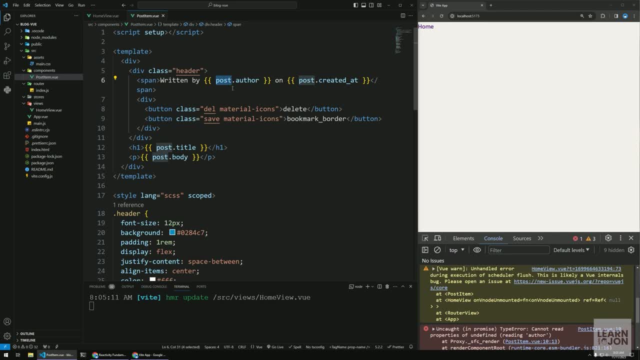 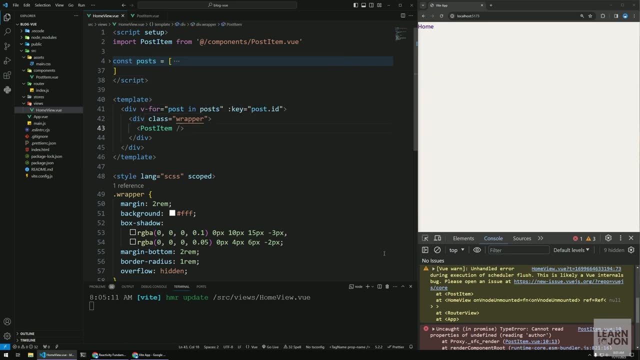 a post attribute or a post variable of property doesn't exist. here you can see that post is actually in our home component. so we need to find a way to communicate from the parent to the child. we need to find a way to send this post back to the child, and we can do so by using props. 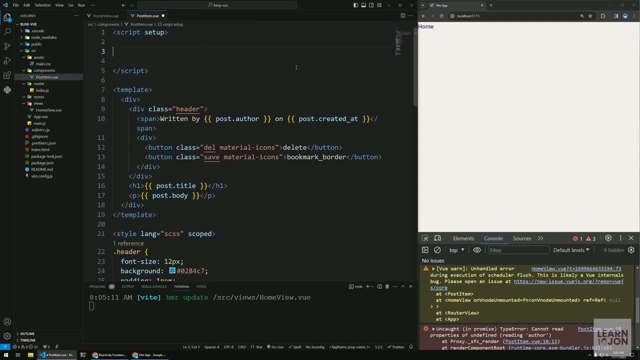 on the child component. we can define props by using the define prop method. now this define props. we can pass an array into this with all the error, with all the props we want to use. so i'm looking for a post so i can pass it in an array as a text. now this component. 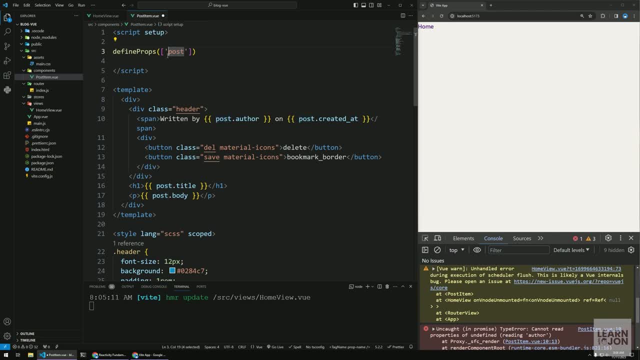 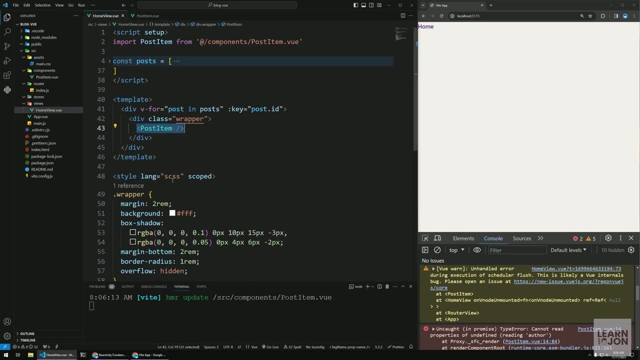 is expecting a prop named post. this is not the ideal way, but i'm just going to show you and then show you the other way. going back to the home view on the component, on our custom component, i'm going to close this style tag, by the way, it's confusing. so now we can pass that post prop just. 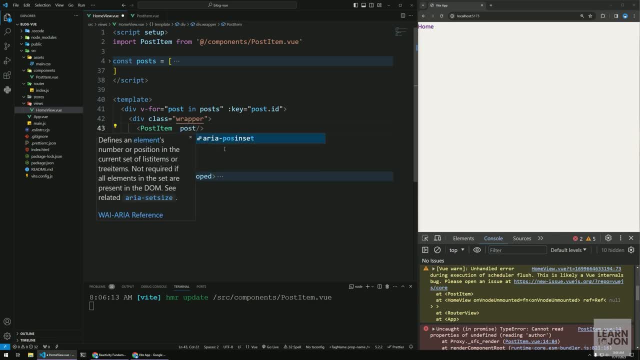 like an html attribute so i can say post and what i'm going to bind to this one is that post up here, because we are looping through that posts array. 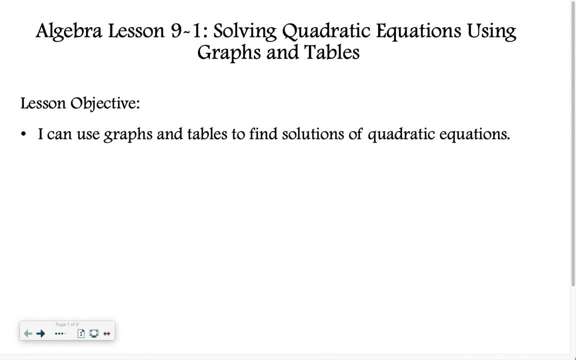 Hello class, welcome to Algebra Lesson 9-1,, which is all about solving quadratic equations using graphs and tables. By the end of this lesson, you should be able to use graphs and tables to find solutions of quadratic equations. Now a quick little side note. these videos I know go. I put them on YouTube. 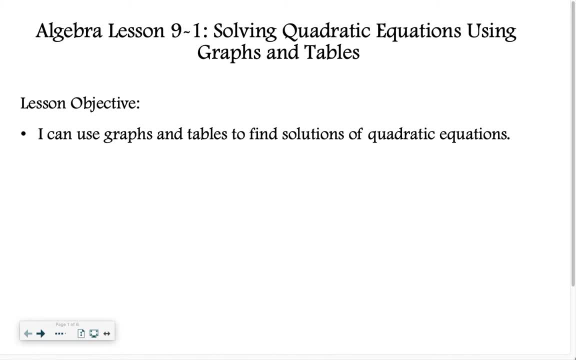 If you're someone that is not my student and you're watching this video and hoping I'll teach you how to use a graphing calculator to solve these, that is not what I'll be doing in this video, because my students don't have those yet. 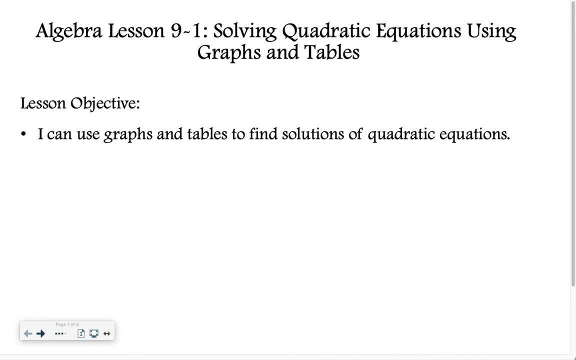 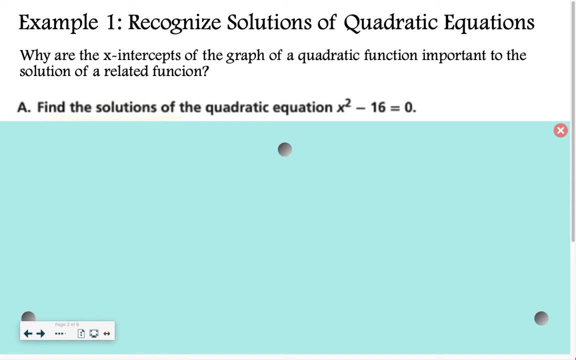 Okay, so this video is not for you. if you're someone looking to use a graphing calculator, All right, let's jump right into example one, recognizing solutions of quadratic equations. So why are the x-intercepts? remember, intercept means where it crosses something, right? 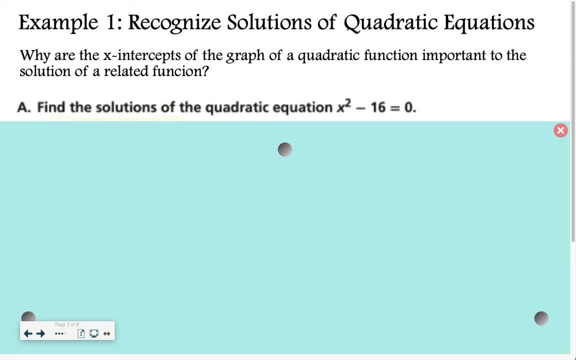 So an x-intercept is where it crosses the x-axis on a graph. okay, So why are the x-intercepts of a graph of a quadratic function important To the solution of the related function? Sorry, I just realized that there is a little typo there.